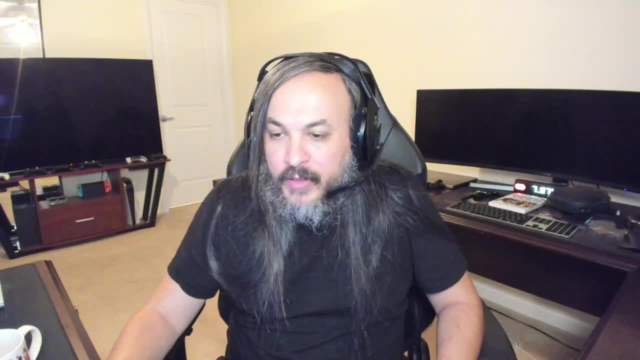 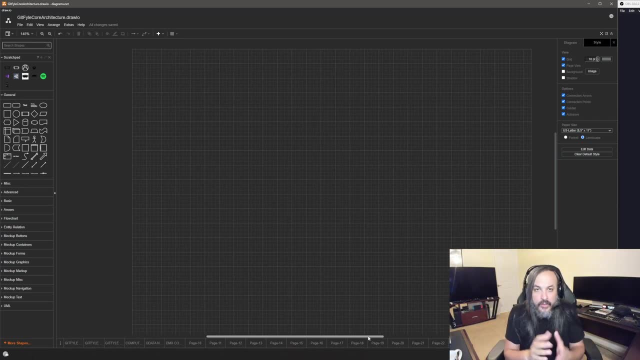 So, for people who are not familiar with what the standard is, it's basically a structure or a pattern that helps you build maintainable software. maintainable simple software that stays at level zero, as I call it, which basically means that anybody, no matter how many years of experience they have, 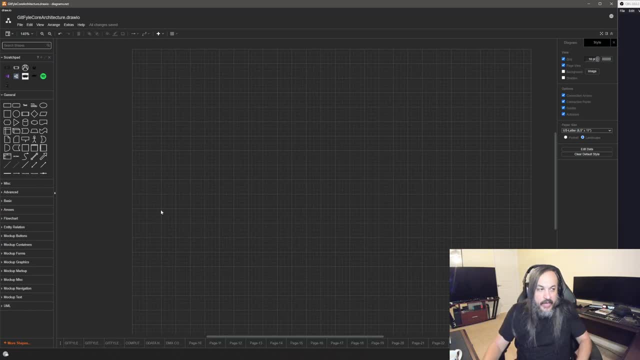 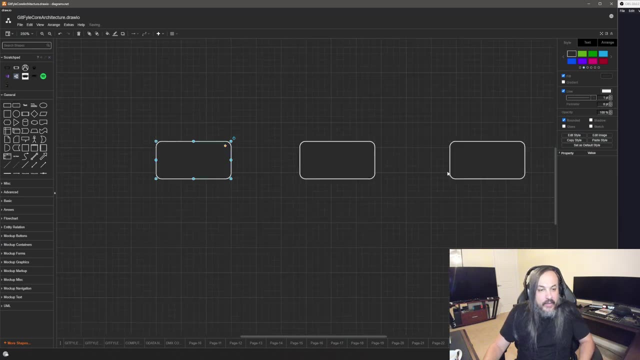 they can come in and actually maintain your system and be able to kind of understand it. The standard is built on a theory called the tri-nature of everything And what this theory, you know, dictates like really, really quick, because there's a whole book and I'm going to kind of drop a link in the video description, just so you know. 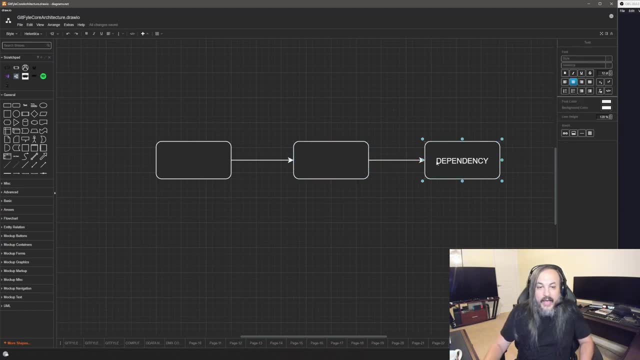 The theory says any system out there, software or not, has either dependencies and purposes and exposures, right? So in your typical, If you're building a simple software or an API or whatever, you're going to have a broker that talks to a database, for instance, and then you have a service that's kind of doing all the business logic and validation. 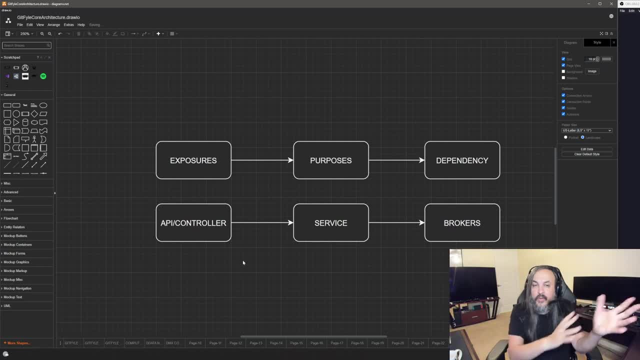 Maybe you have an API or a controller you know that basically exposes, you know, all that work of the service to the outside world. There's a huge theory behind this, a big community behind this. I'll drop all the links down there just to kind of, you know, give you that kind of idea of what the standard is and how people kind of build systems you know in work. 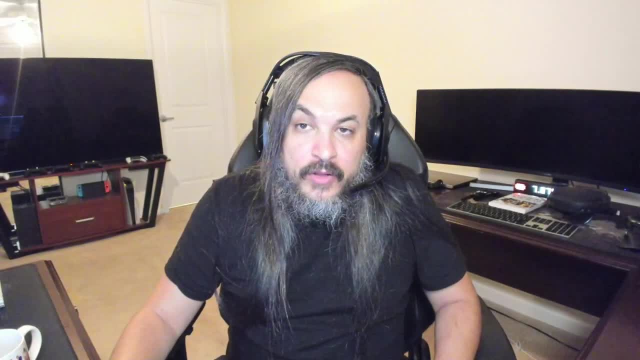 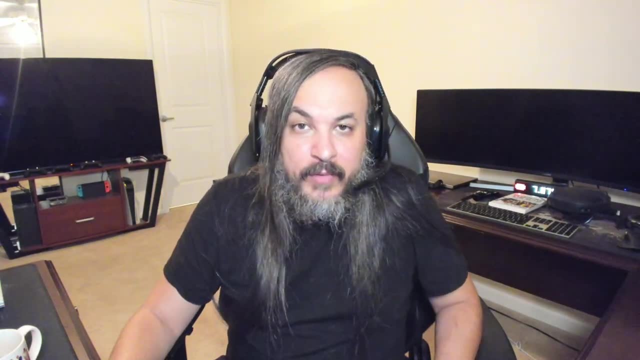 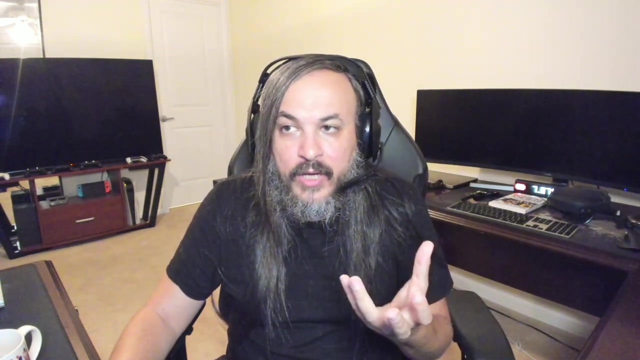 One particular way or another. This language that I'm going to be experimenting with, though, is very special. It's very near and dear to my heart, because, you know, this is one of the languages that I've actually- Not a lot of people probably know this, but I actually started, you know, kind of formalizing and building some ideas and concepts around. you know kind of advocating for the engineering standards from working with Scala. 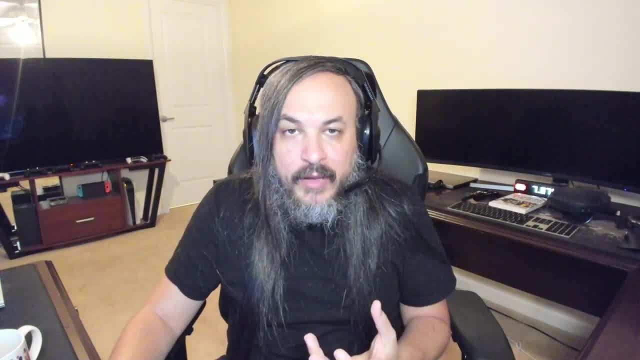 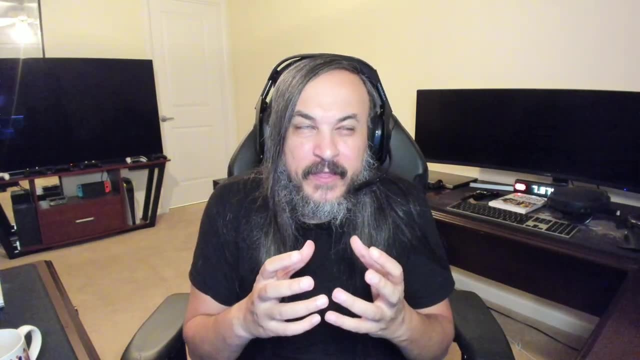 Scala is an amazing, amazing programming language. It basically helps you and gives you the ability to kind of think, You feel You feel like you're thinking. It kind of gives you like this weird feeling that you are truly a computer scientist, right. 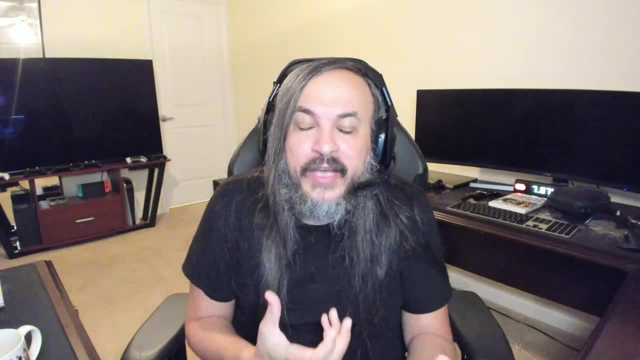 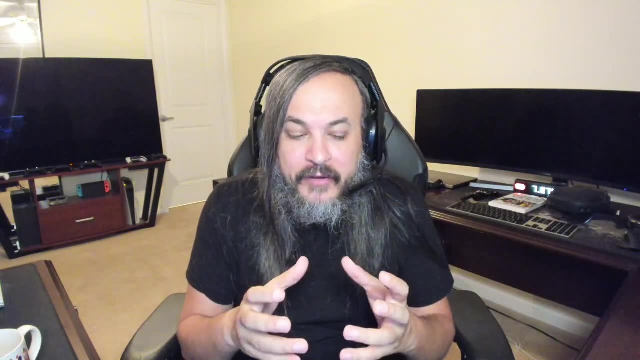 It's a functional programming language that kind of respects your brain, It respects your intellect, It kind of plays with you in a certain way, as long as you can kind of wrap your mind around some of the ideas you know and some of the functional ideas that it's trying to implement. 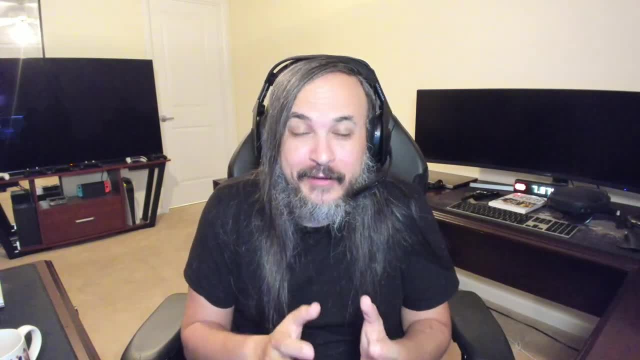 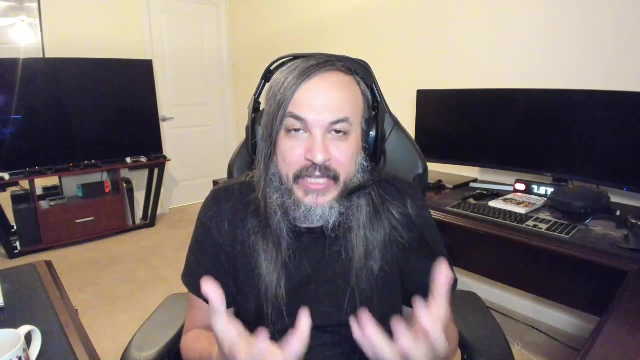 It's also object-oriented. It's actually a. It's a cute language And you know you can quote me on this. Scala is really cute because it kind of gives you this kind of feeling that you don't have to write code, you know if you don't need to. 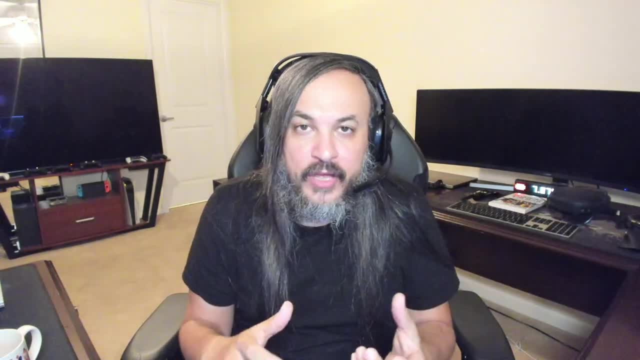 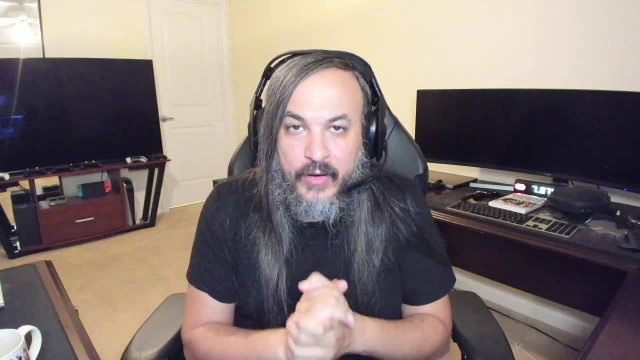 You know, very short, precise, simple thing. Some of it I really wish we had in C-sharp, hopefully soon. You know we can kind of adapt to these patterns, but it's definitely a great programming language. So let me just tell you what I'm going to do here today. 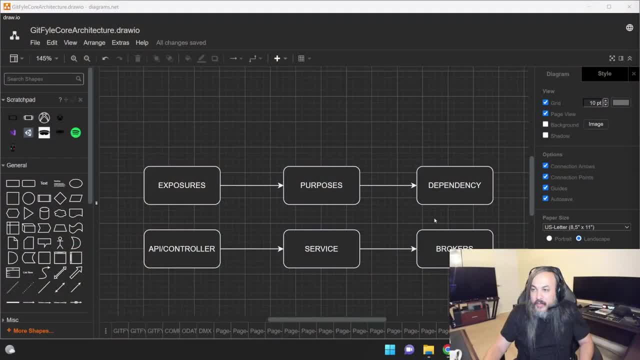 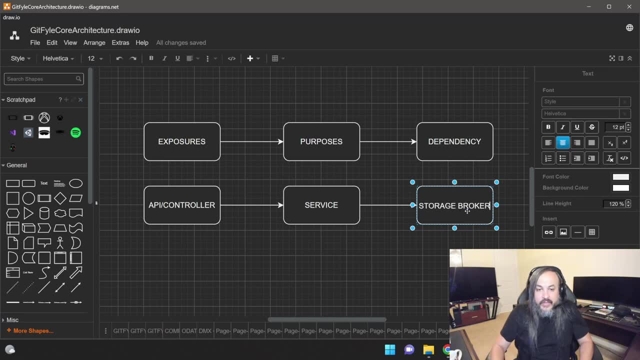 I'm going to implement- just like I did with Go, You know I'm going to- I'm going to implement a simple program that basically goes and says: here is a storage broker for a student service and here's a student service, right. 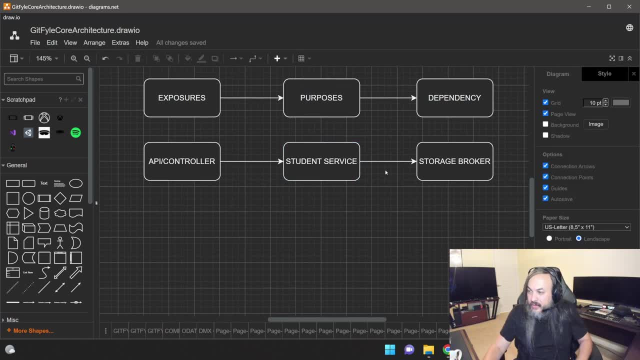 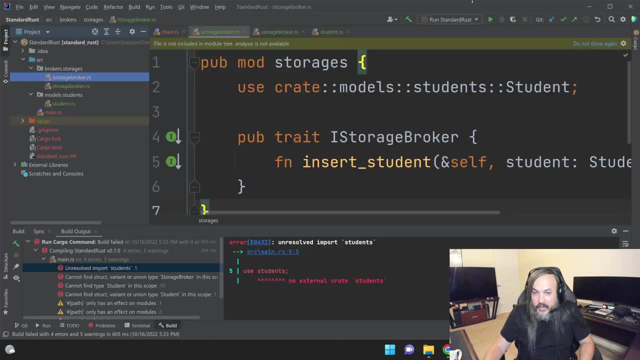 And then we're going to go and write a unit test for these two things. right, A simple unit test that can kind of show us how things work. One of the things that we can use here is IntelliJ. This is me playing around with Rust. 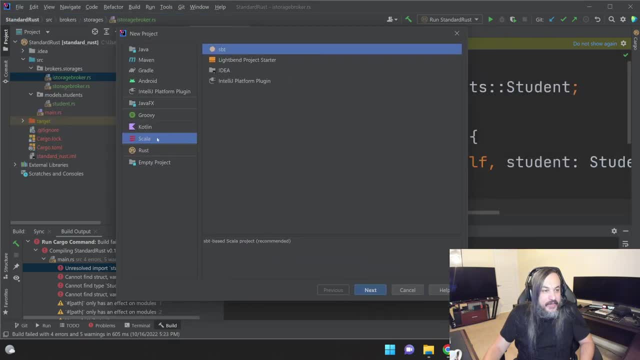 You don't have to worry about that, Let's create a new project here. So here it is. So you select Scala, And then I selected SBT- I think it stands for Scala Build Task, or something like that- And then I'm going to go here and say Standard Scala. 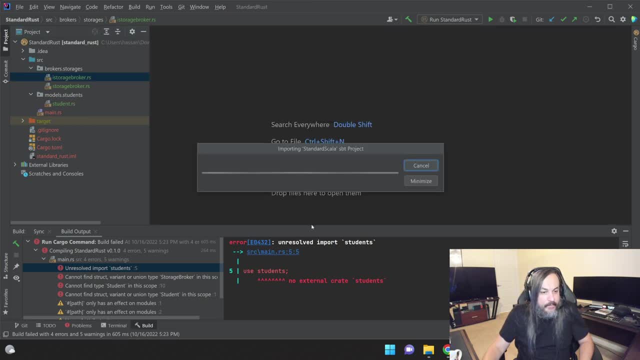 Yeah, let's open it in this window, Why not? Okay, here we go. I hope it kind of cleans up all the Rust stuff that I'm dealing with. Rust is just a whole different beast that you kind of need to kind of think about and explore. 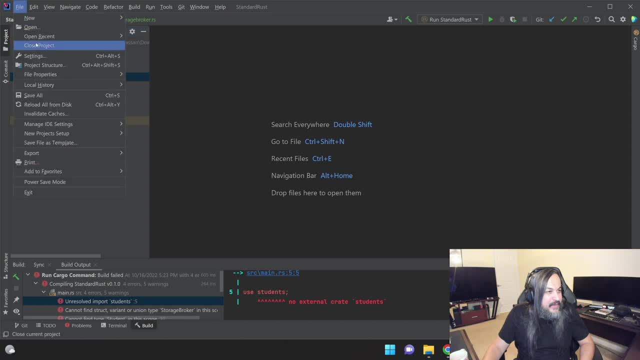 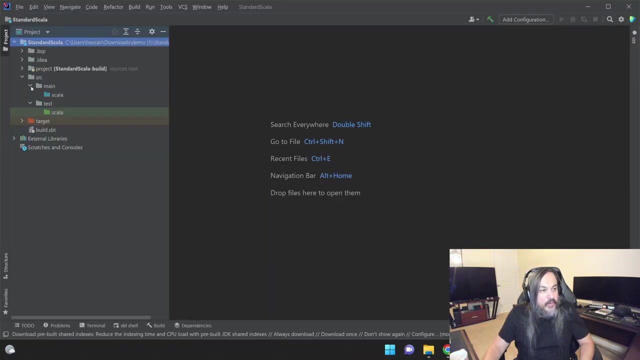 Let's see here. Did it actually open it? Let's see, I should have opened it in another Open recent Scala standard. Yeah, let's open it in a new window. Let's just avoid the traffic, Okay. so when you create a new Scala program, you have two things here. 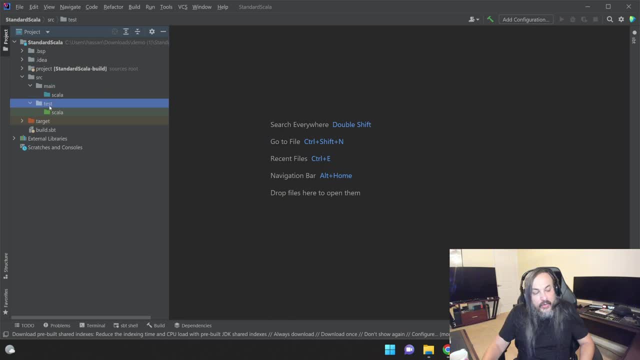 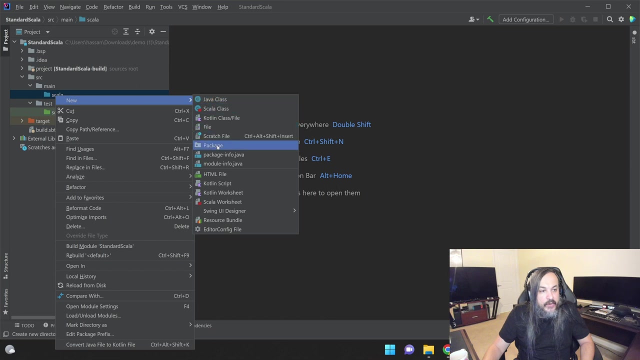 You have Scala, Scala, you have a test and main right. So what we're going to do here, I'm going to start kind of pulling my all my folders and everything inside that kind of main folder. I think you can distribute it anywhere you want. but let's just start from here and create a package. 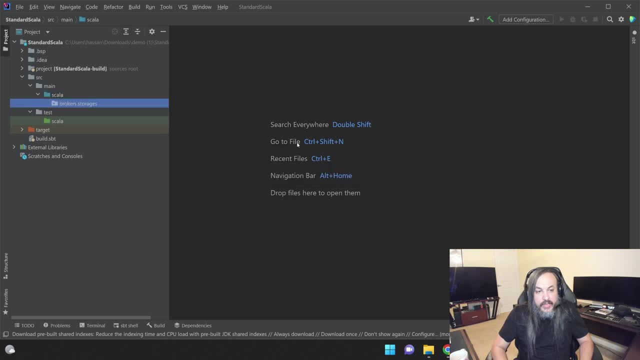 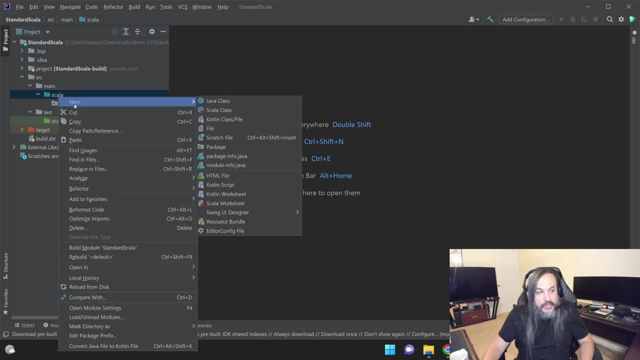 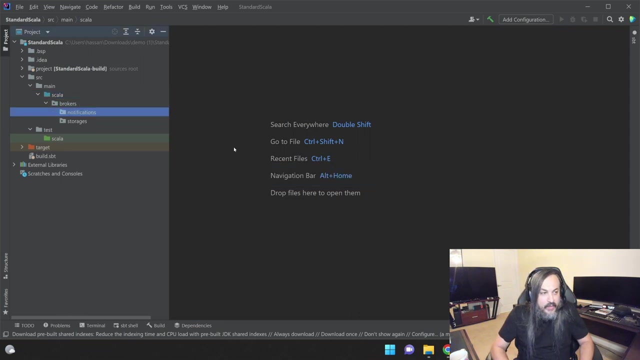 I'm going to call it BrokersStorages. So here's another cool thing that I don't see in NET or Visual Studio. See, I did BrokersStorages. So that means if I have a different kind of broker which is BrokersLet's say I don't know notifications like this, it will. 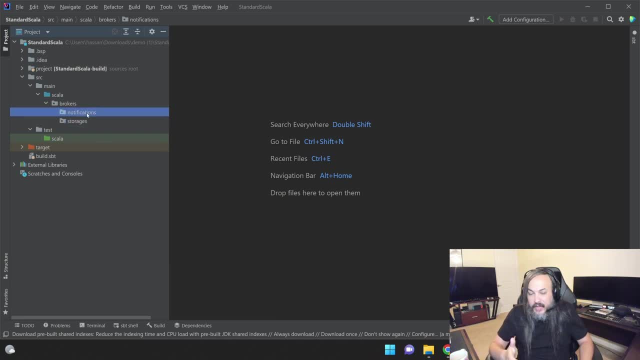 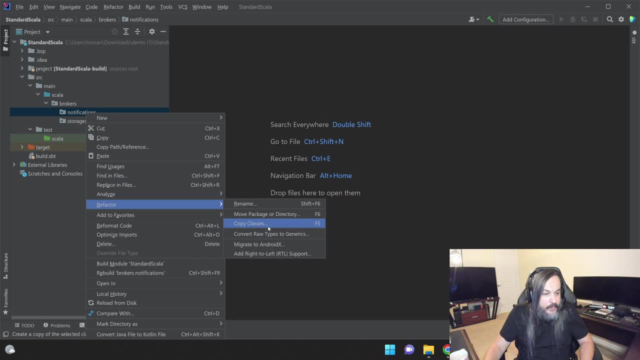 nest very nicely, And I think this is an IntelliJ thing. You know, this is not specifically a Scala thing, It's an IntelliJ thing which is pretty cool. Let's delete this guy. We don't need it here. How do you? how do you get rid of that? 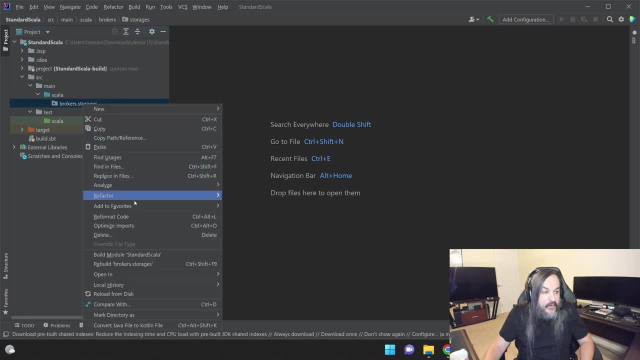 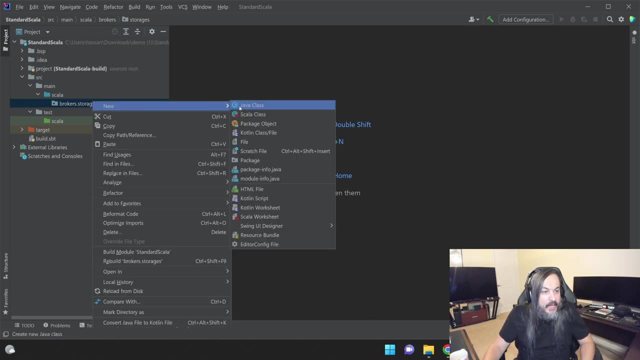 Delete. There you go. One thing that's not cool is that with refactor you can delete a file from refactor, but you can't delete the directory from refactor, which is kind of weird to me. I'm going to violate some of Scala rules in here. 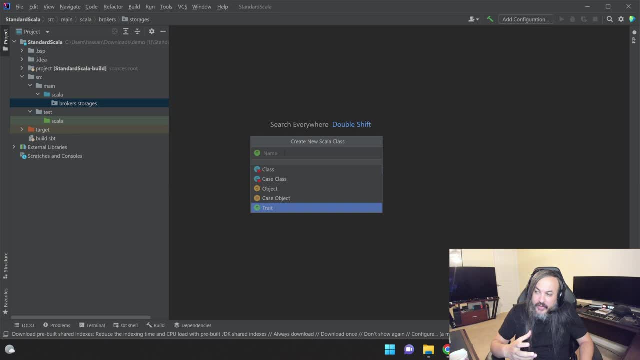 I might go and say so I need a trait. They don't really have A naming convention for traits. Traits is basically the interface, right. And since most of the audience, the people I'm talking to, are NET folks, it's probably better if I go and say: I storage broker the way we name you know things in NET, so people kind of understand where I'm coming from here. 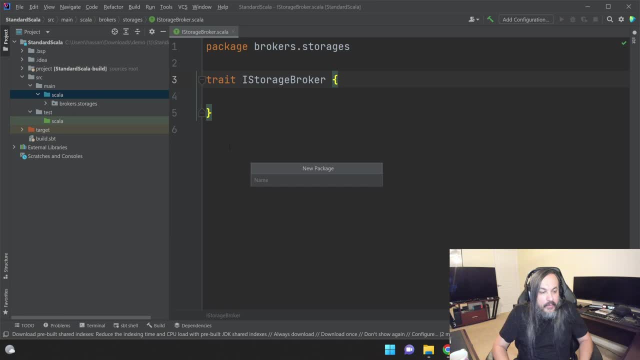 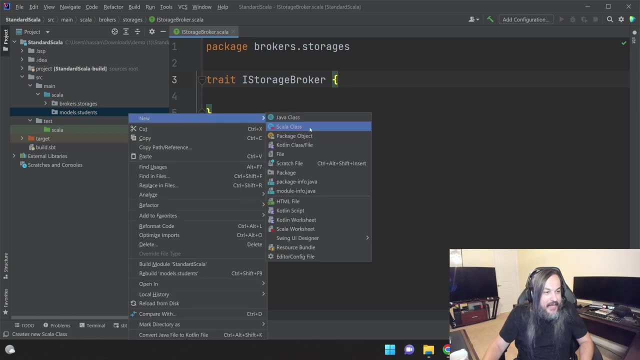 OK, I also need models. Let's go and create a bunch of models, or his models, And then, under models, I'm going to go and create students. I should- I should have just got that leverage- and then I'm going to create a Scala class and I'm going to call it student. 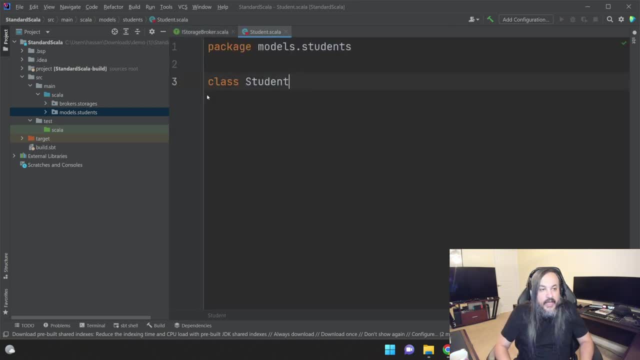 So that's my student. Watch how beautiful this is. You can go here and say: for my student class. I can just go and say: it's a variable, that's a name, that's a string and that's your input parameters, That's it. 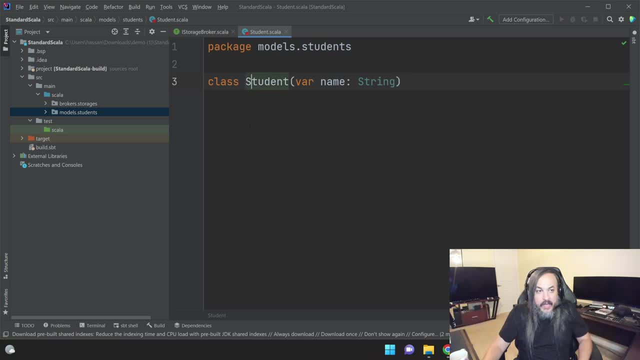 You just created a class just like that. How crazy is that. And for for the Scala gurus out there. you know again. you know, I put these videos. As far as I remember it's it's been a long time. 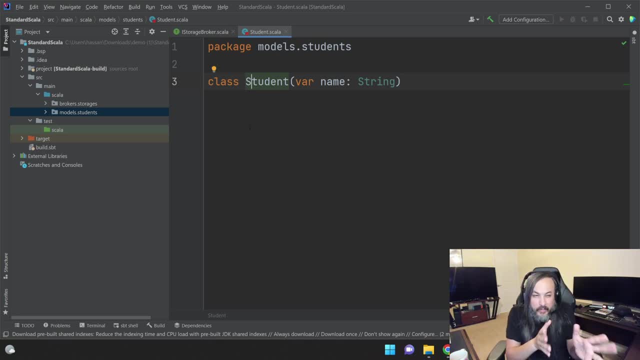 I actually worked with Scala, but I think you know this is the proper way to do it, something like that. So this here basically is the equivalent of C sharp. when you go and say public class students and then you go and say public string name gets it. see, all that work that I just did. 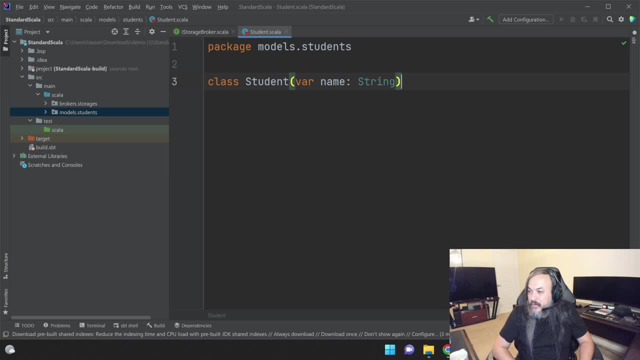 You can just do all of that very easily in Scala. just by doing that right, Someone might say, well, I want to do more things. Of course, You can go here and do this and you can define functions and you can do setters and getters and whatever you need. 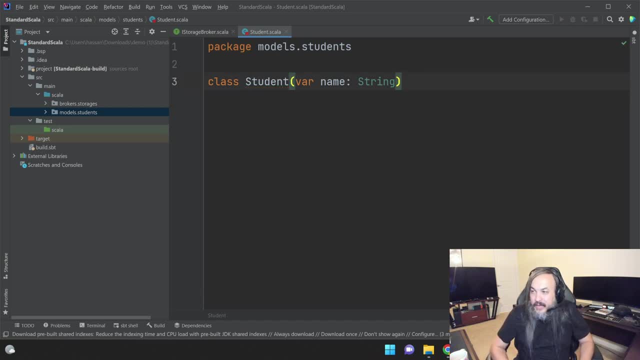 It's kind of. this is again like I said to you, it's a cute language, right. It kind of works with you to get your idea out the door as soon as, as soon, as fast as possible, while maintaining a sense of beauty, you know, to the language itself. 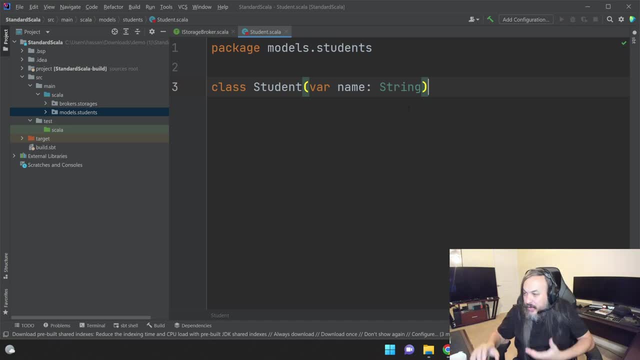 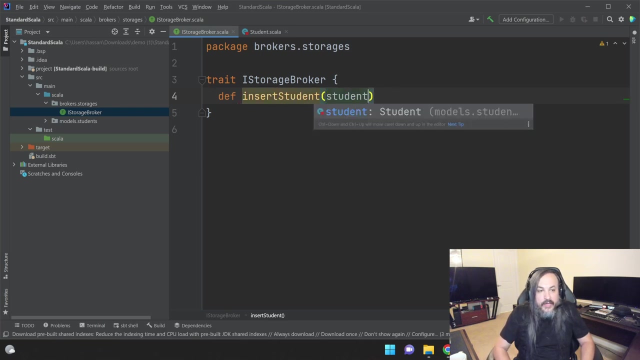 It does maintain a sense of beauty of how it expresses idea and kind of mirror your ideas and all that. OK, let's go back to the storage broker in here. This storage broker needs to define a A function called insert students, Right, and this insert student function will take in a student variable of type student. 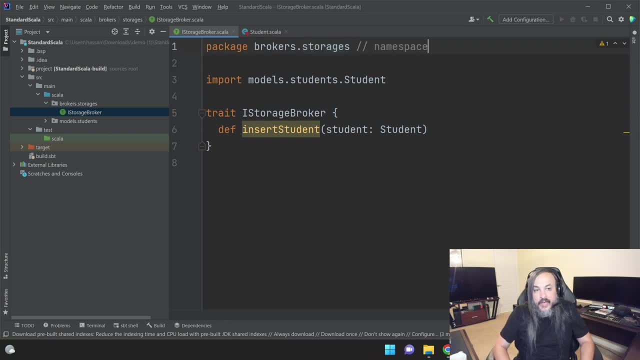 Just like that. you see the package. the package is basically equivalent of a namespace in the dot net world and then the import is the equivalent of using Right. so let's say someone might hear say, OK, I don't want, I want all the models under students. so you can do underscore like this: 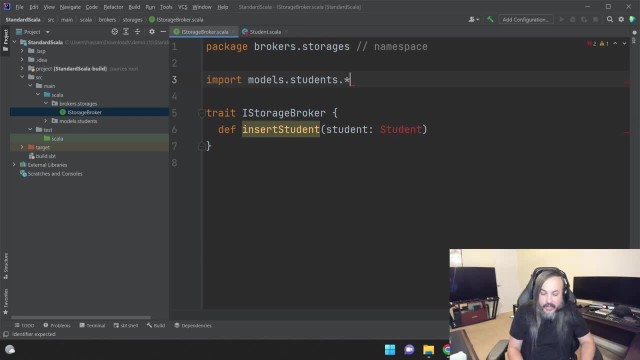 So now you're pulling everything under And I think in in Java you would do this, but in Scala you would do something like this. By the way, Scala, I think, is running on JVM as well. This way it plays with Java very well. 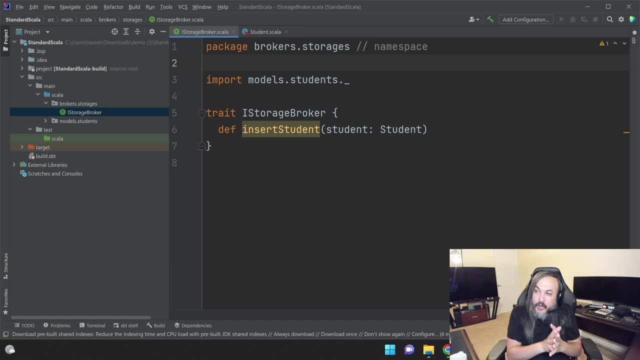 It's Java's smart cousin. That's what Scala is. The best way I could describe it is Java's smart, smart cousin. OK, anyway, how do you say that this interface returns something? you go here and say, you know, kind of a colon, and then this is how it's returning things. 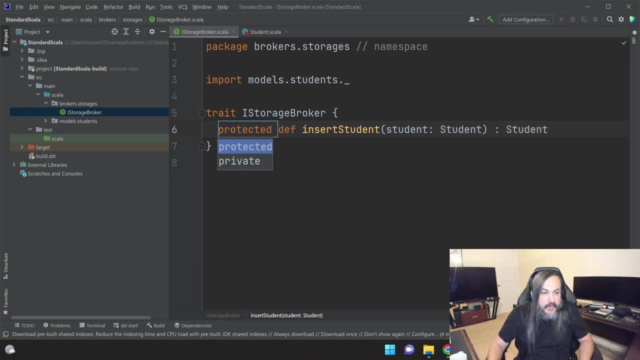 I think Alt Enter is how you- No, I don't want to do that. Yeah, Alt Enter in IntelliJ, or at least the version that I'm using, is how you're basically doing this, This nice little number in here. OK, so that's an interface. 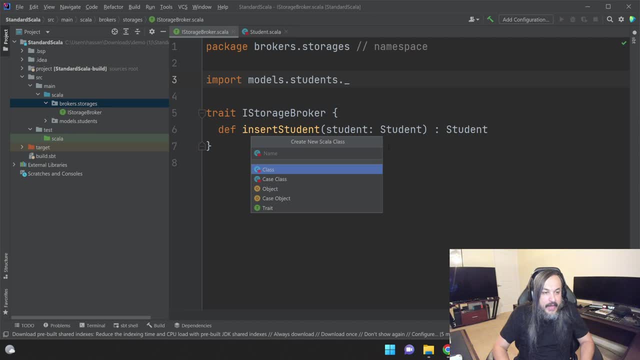 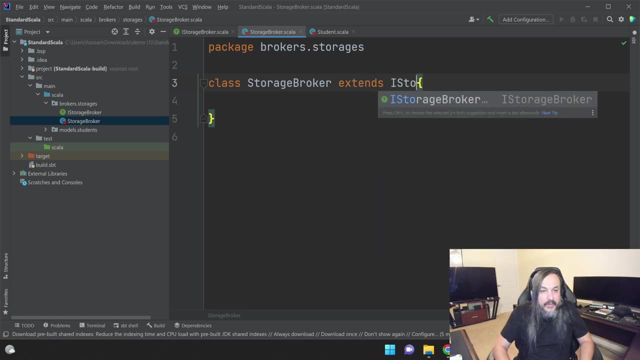 Let's go create an implementation of that interface. So let's go here and say: this is a class, It's called storage broker, And then in here you can go and say: extends, I storage broker. And then if you do, if you do an Alt, Enter in here. 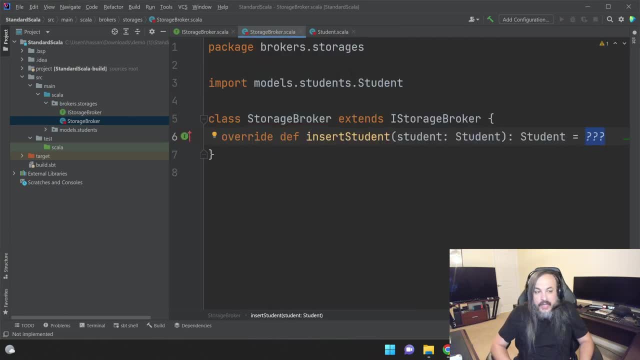 It will say: go ahead and implement the method. Boom, just like that. Look at this. You'll find a lot of these things here in Scala, You'll see, like question mark question. This basically means there's nothing here. I don't know what's coming, you know, and I think it's pretty cute. 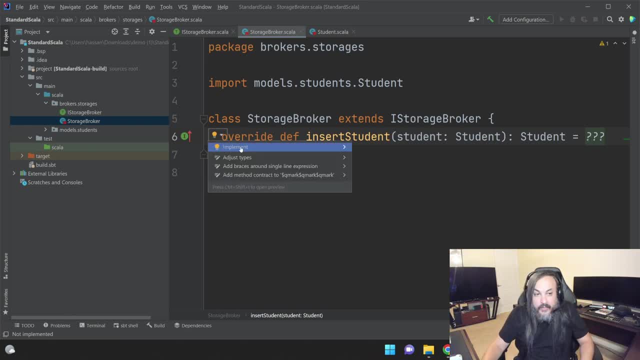 I told you before, this is actually really cool. What are these question marks? It basically says, hey, I think an implementation is required in here. right, These three question marks that basically say there's nothing in here yet, because this is a broker. 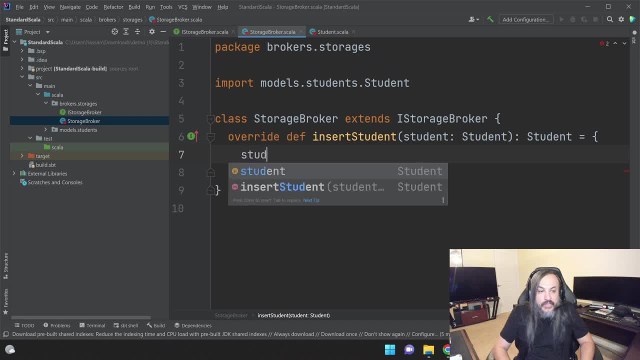 What I'm going to do. I'm going to go And say this broker just is going to return the student. Here's another cool thing: You don't have to say return like that. You could just say student, and it knows exactly what you're trying to say. 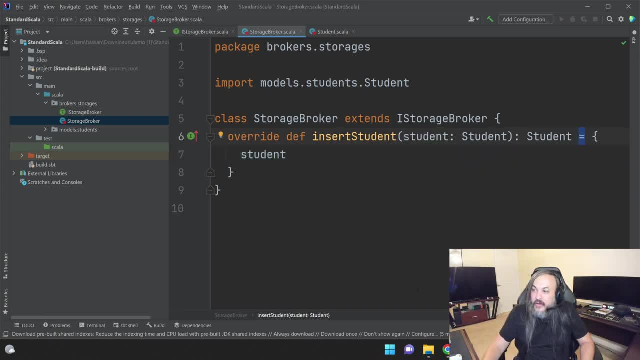 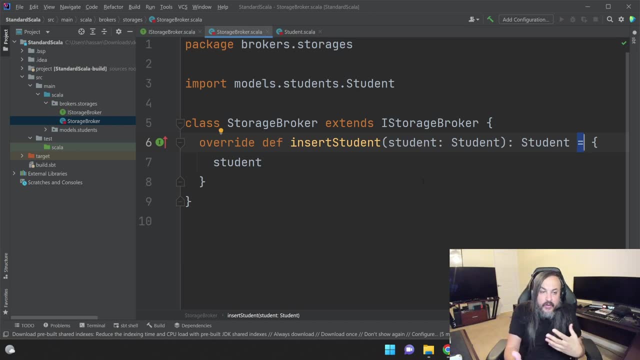 One thing I don't like: this little equal is unnecessary. but it's a functional language. It thinks of everything as values. I think it thinks of everything as values and references and functions. So it- I guess you know how they decided to do this- is to equate every function. 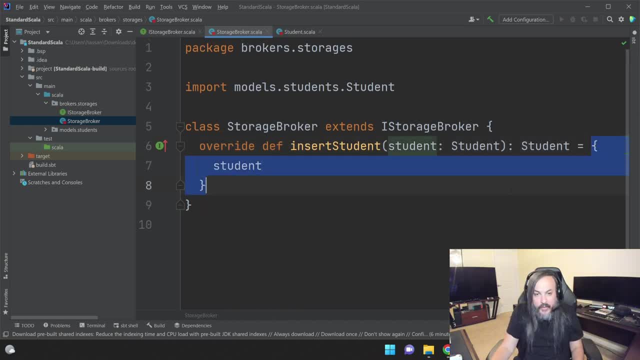 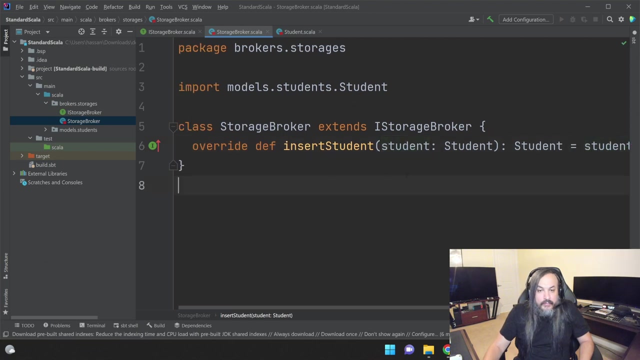 To like. I'm assuming that this is from here to here. This is a function or an anonymous function in some way. I don't know, I could be wrong. Okay, so that means I could just do this. Then I could just go like this and say: student, and that will work too right. 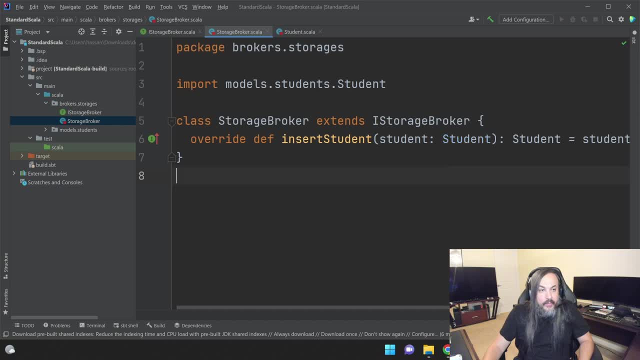 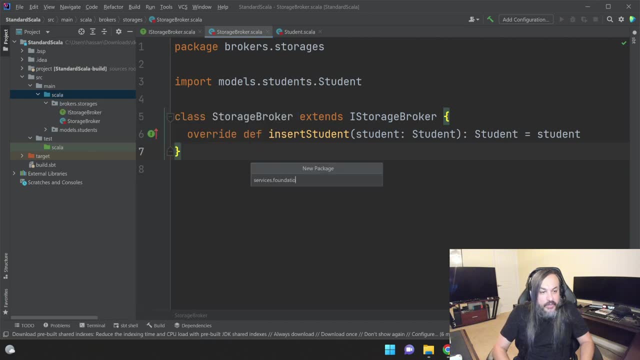 That's pretty cool. Uh, okay, so that's the implementation of this. I have a storage broker. Let's go ahead and create a service. So here's services, dot foundations, dot Students, just like that. and then I'm going to create an interface. 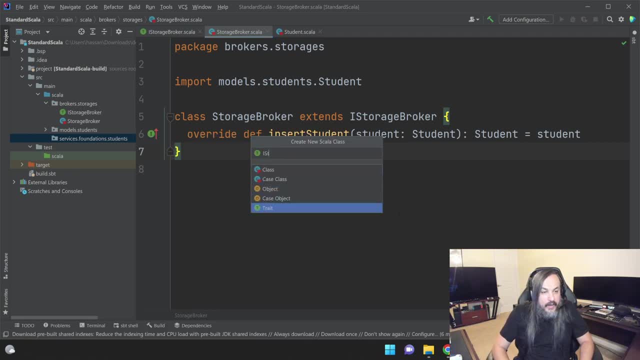 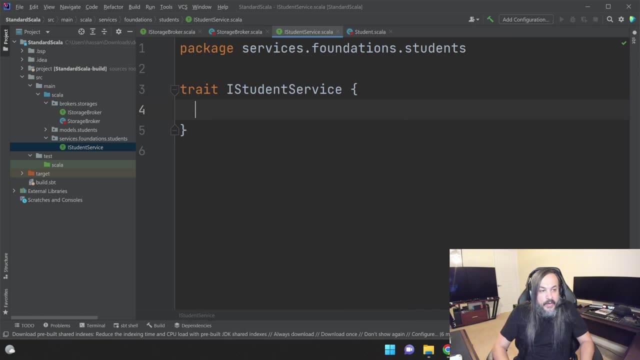 So here is a trait, and that's I student service. There you go, And my I student service requires a function called add student that takes in student as an input parameter. Here's alt enter: pull in, There you go, Alt enter And then it. it should return a student model. 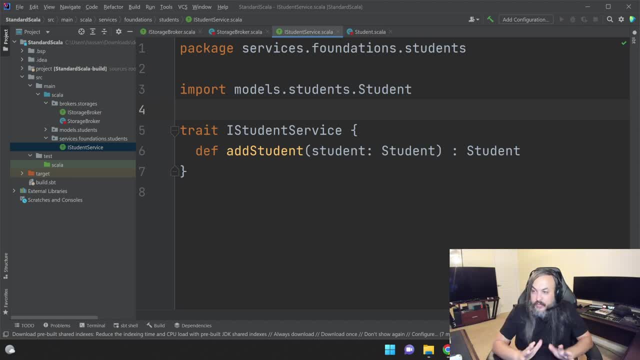 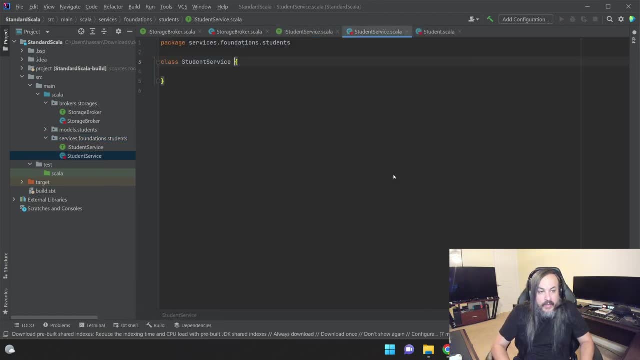 So that's an interface. See it's, it's, it's amazing language, beautiful language, It's playing with you, right, Let's add an implementation for this. So this is a student service like this, And then I hate that. 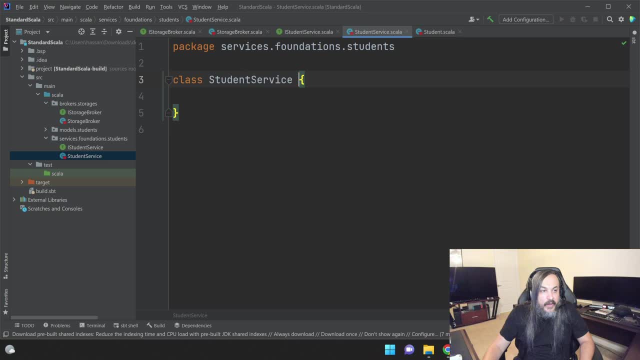 I have to kind of zoom in with every file. That's kind of dumb. There must be a way that you can do this nicely. How do you inject a dependency in a student service? You just go here and say this is my storage broker. 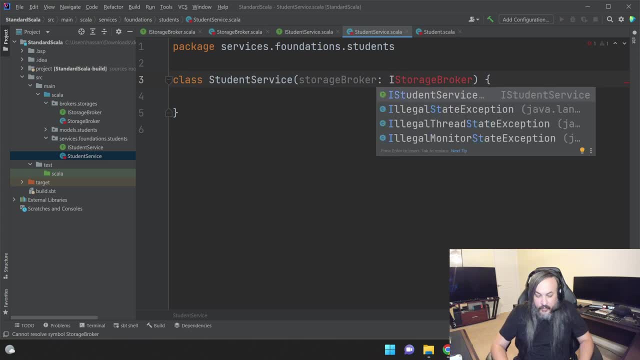 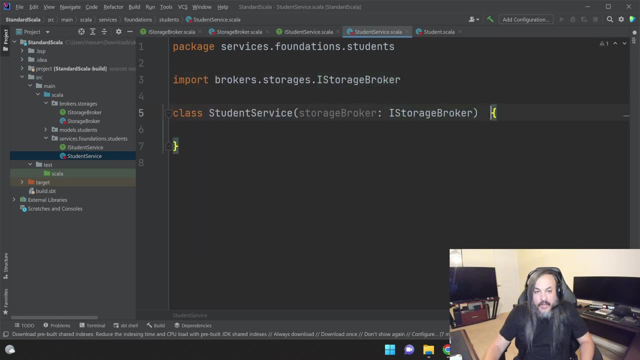 Right, And that guy requires that interface. So my I storage broker in here Will basically pull in this as a dependency. but it also extends- That's your equivalent of implement- I student service. Okay, so now this guy is complaining. It's saying I don't have an implementation. 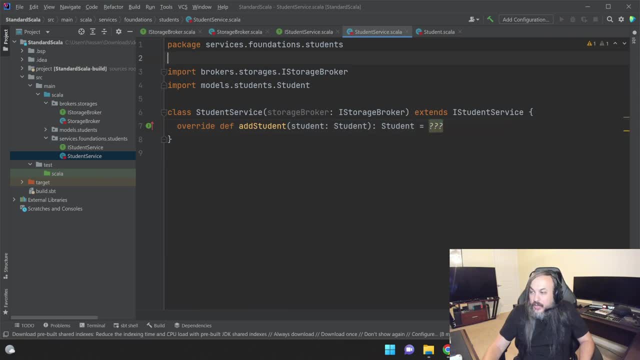 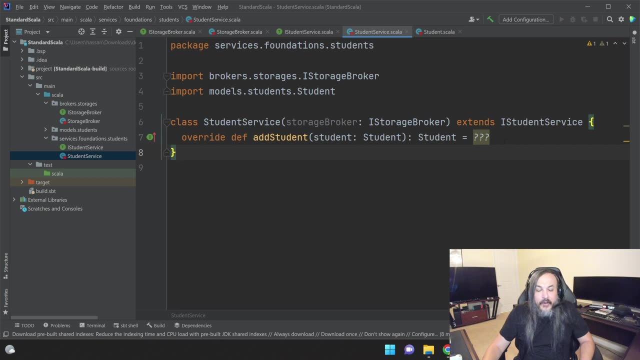 Here's your implementation and we are intentionally not going to add an implementation there. I'm going to go here and say: yep, you know, this is my implementation Question for a question mark. you know, whatever that means, We'll see what that means in a second. 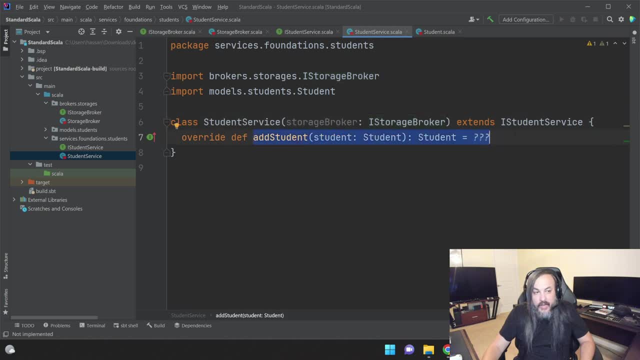 Okay. so I can't add, because this is test-driven approach. I can't really add a, I can't add an implementation to this, unless I have a failing test that tells me you need to add an implementation to this, Right? So that brings us down to the second folder down here. 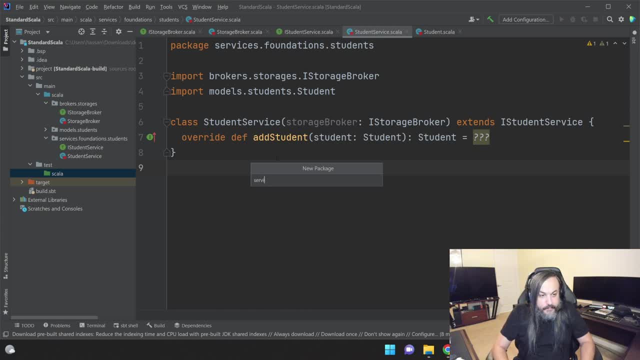 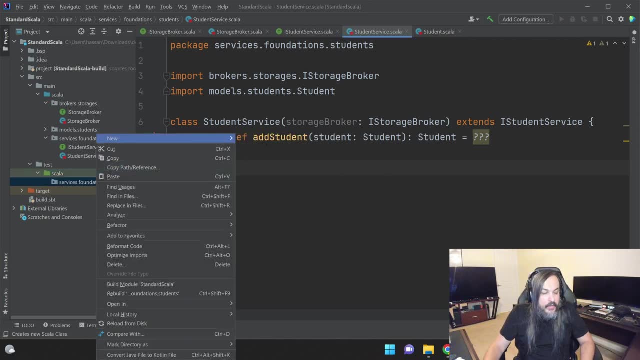 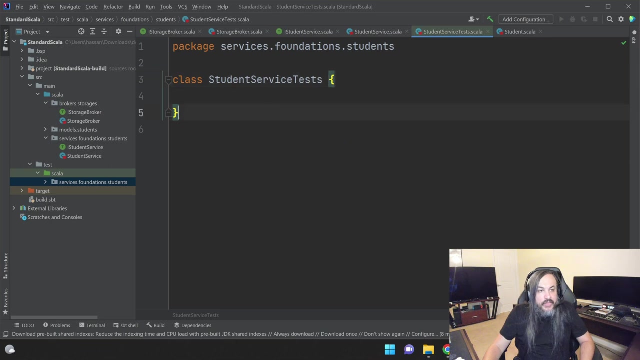 I'm going to go here and create a folder called services, Foundations- students. and then I'm going to create just a tiny nice file in here. I'm going to call it a student service test Scala. super forgiving, with naming conventions- Super cute. 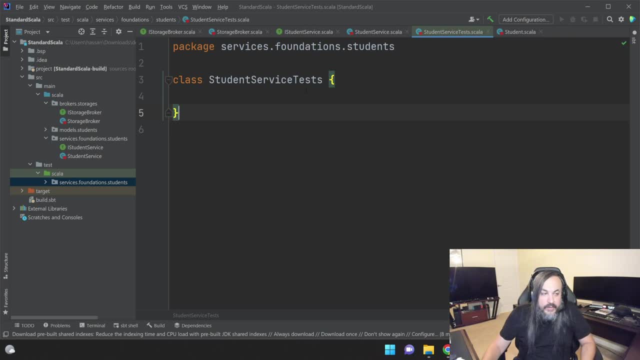 It will let you kind of do whatever you want to do with your naming conventions, Unlike go, which dictate that your test has to start with the with the name prefix. craziness I don't need, you know it's crazy, So okay. 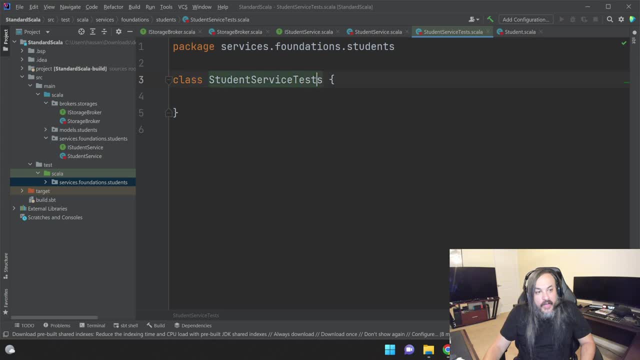 So so I have this class and this is my test and whatnot. We need something called fun sweet and makito. fun Sweet and makito is basically like us pulling a mock, mock dotnet and your MS test or X unit and all that kind of stuff in the in the dotnet world. 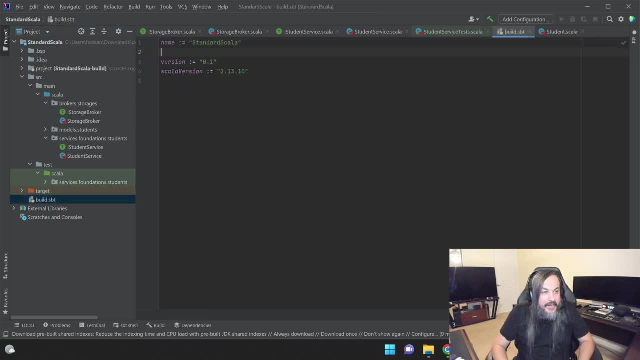 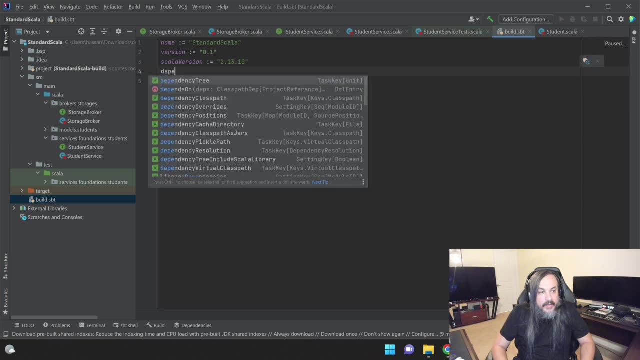 How do we go about doing that? There is that there is this thing called a, a build file. So this is build at SBT and you basically go and basically add dependencies, Right. So you go and say: I'm not going to pretend that, I know these. 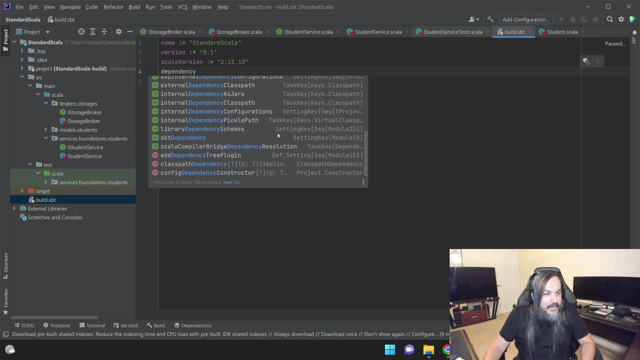 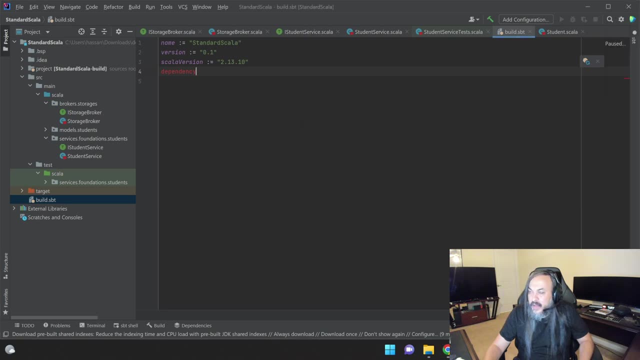 I'm just going to try and find it off the bat. It's supposed to kind of help you out, But of course I have a couple of sites in here that will tell me: hey, here's what you want to add, and all that. 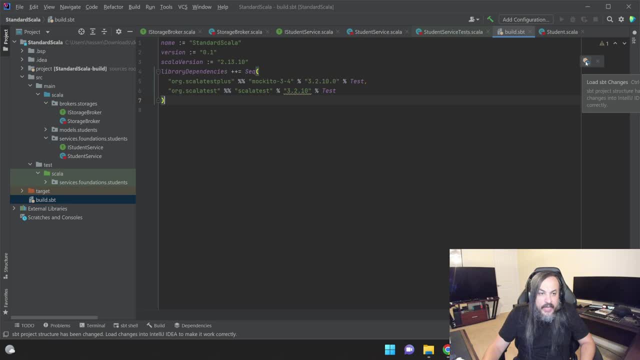 There it is. So you basically go like this: You see that little tiny thing that's showing on the on the right side up here. This is the guy that's going to pull these packages in. There's also this nice thing in here where you can go and say: I'm doing control period because of Visual Studio. 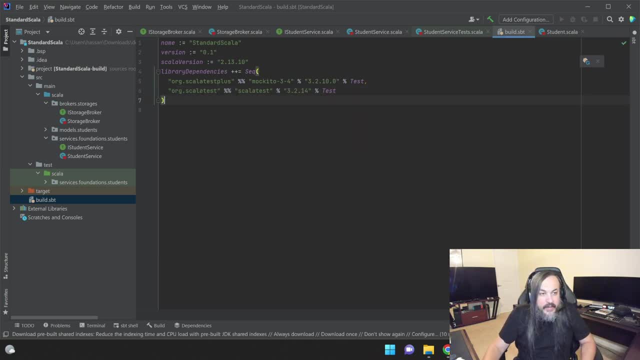 But if you go and say update dependencies, it will update. So this is basically the dependency name, Right, or sorry, the organization and this is the dependency name, And then this is the version of the dependency And I think this is what you're targeting. 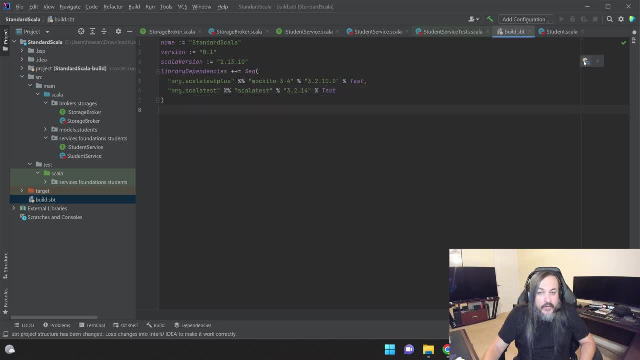 I don't remember. I don't remember what this is, but we need to pull these dependencies. You'll see a whole bunch of things. This, this little side here of the world is going to explode. You're going to see all these libraries being pulled. 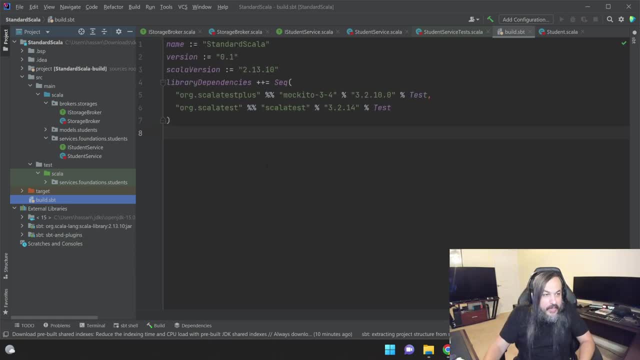 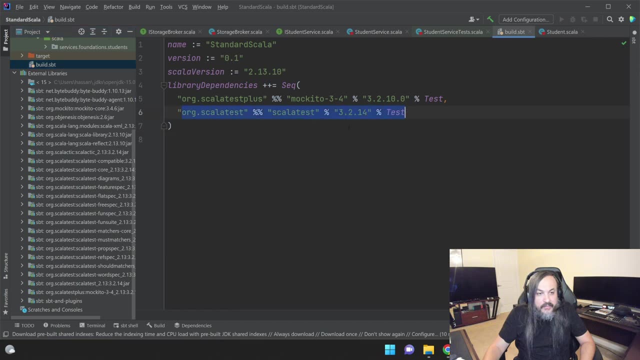 I think from Maven. I don't know what Artifactory they're using. It's been a long time, but look, it basically pulled all these dependencies for you. So this is the core Scala test framework, And then you also have the Makito, and Makito is what I use to kind of mock these dependencies. 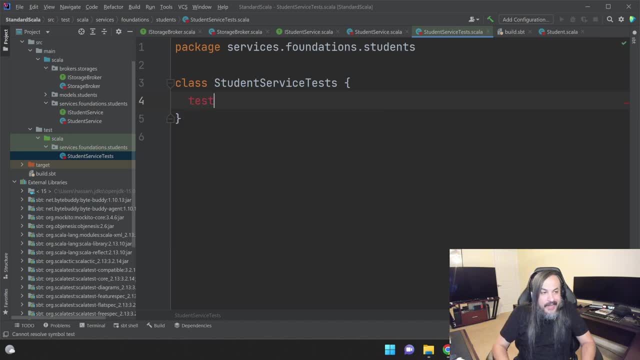 Okay, let's do this, So I can go here now and say, test, right, And it's going to complain if I do control period. Oh, this guy needs to extend. Fun, sweet Like this. There you go, And then I can go here and say test. 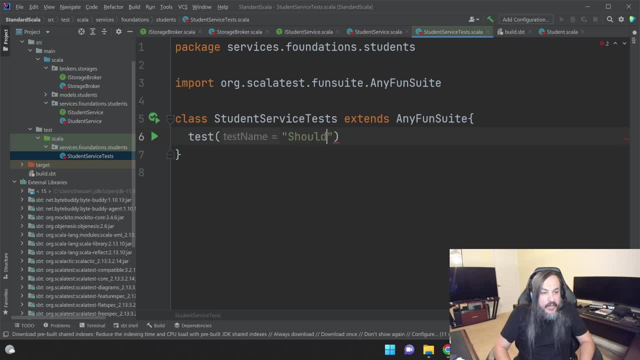 There you go, And then we can basically say should add students, Or something like that. This is how we basically write our tests and dot net, at least you know, with the standard community and all that. I don't like these automated, kind of automatic in the browser, kind of sorry in the editor. 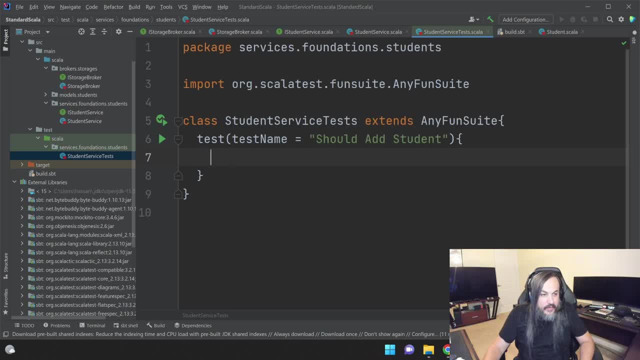 Kind of Adding the variable name. So I'm going to add, I'm going to say: this name is this Okay? so, just like any test, we have a given, We have a win, We have a, then right, and I can go here and say, well, you know, mock up a student for me, right? 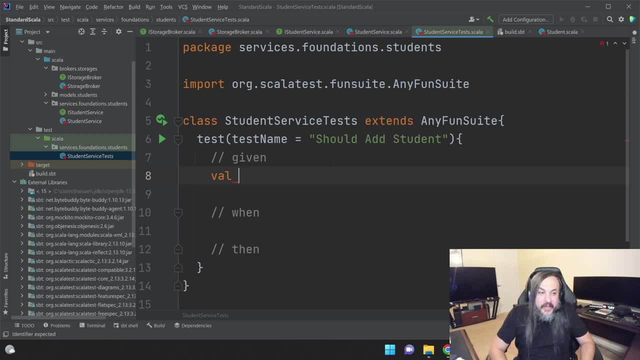 So here's Val. Val is like, how do I explain Val? There's Val and there's VAR, and you can define things if they're- I think it's their, if their final values. You don't have to call them VAR. I think that makes them immutable. 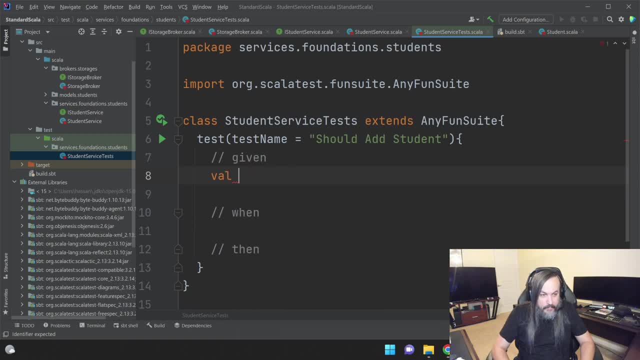 If they're, If I'm not mistaken. So if I go here and say Random student, I can go here and say mock, Now, now it's asking for the thing mock, and then I could pass student here as a dependency. Let's see if it can find it. 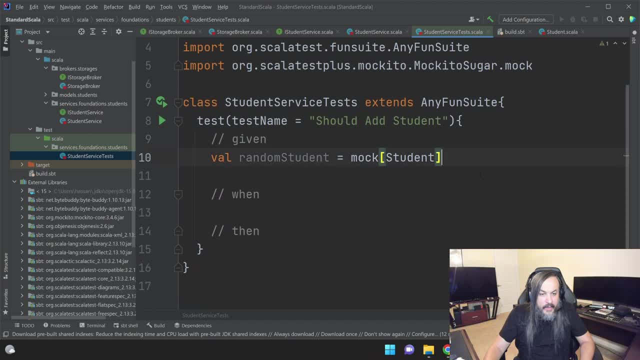 There you go, So here's your student, And then we can go and say: so. does that mean if I go random student dot name equals. is it going to complain? No, I actually don't remember what Val was for. But anyway, here is input students. 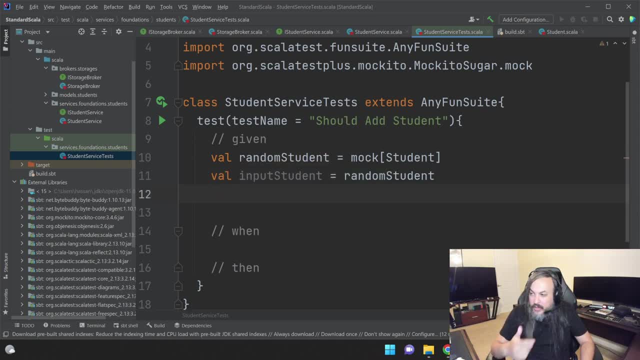 Which is also from this guy. I'm only doing this naming convention because of: like, the naming of the variables plays very well with where you set them up, So it's contextual, even though they're exactly the same values. So this is inserted. student. 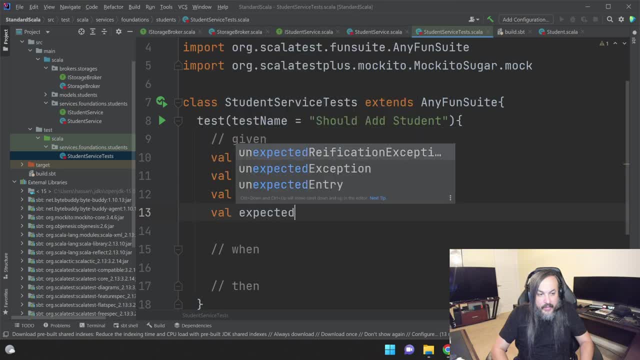 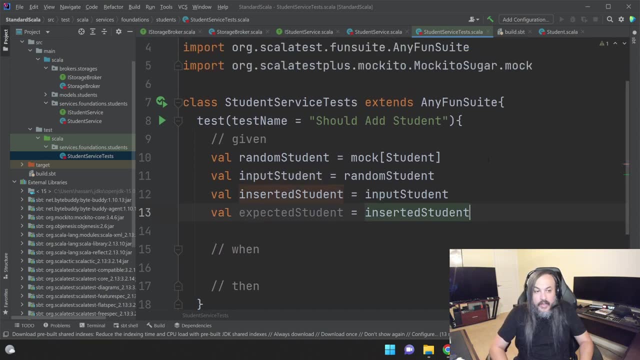 Which comes from input student, and then the last thing is expected Student, which comes from inserted student. They're all the same, Very the same variable. The only difference here is that I am setting them up in a in a particular naming convention, So they fit what I'm trying to do. 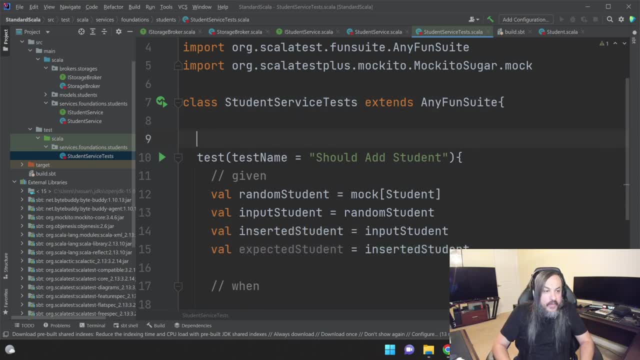 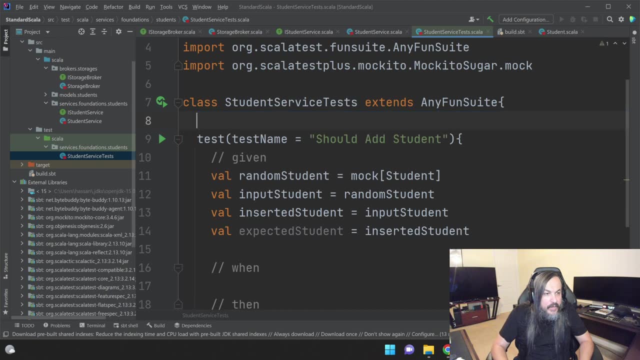 Okay, that's cool. I think there is a thing here called before, And this is not something I have done to prepare for, But I really want to show you like, well, let's just do it here first, and then I'll tell you what we can do with it. 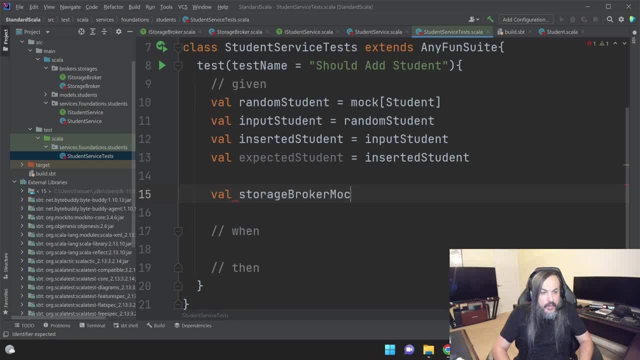 Here's Val. Here is storage broker mock- So his mock. and here is my I storage broker. I marked my storage broker Right and then I also have Val student service. This is what I'm really trying to test, and this is just a new student service. 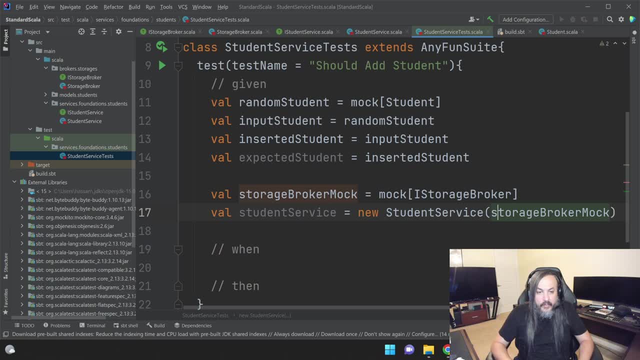 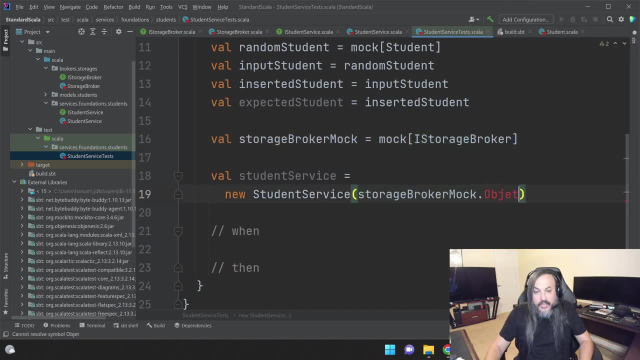 And this student service will take the storage broker mock as an input parameter. Here's the cool thing about this: in dot net You can't really go and say you have to go and say mock dot object like this, which is really ugly. I don't like it in here. 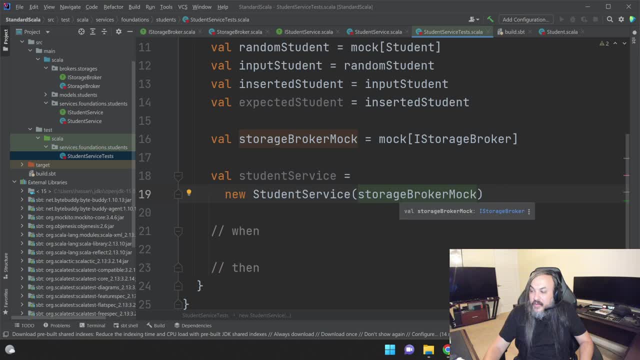 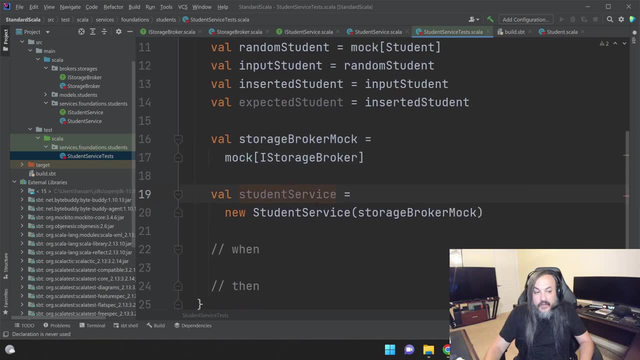 It says: yeah, you mock this, I know that it's a mock, or even though it's still the same value, That's pretty cool. That's pretty cool because that basically means: hey, dude, you know, you don't have to worry about calling an object. 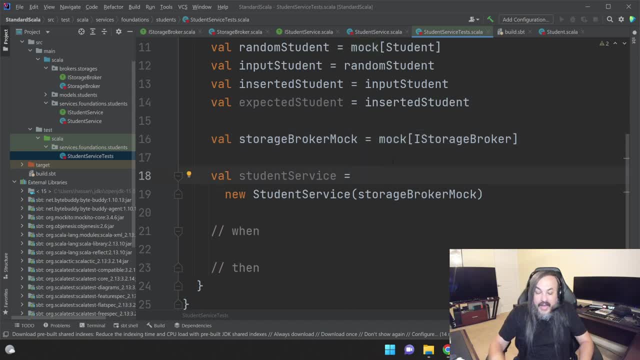 I know this is a mock. It's going to pretend to be. you know that mock is going to have this additional capabilities and functionalities Without you having to say dot object. That's beauty. I love this about Scala. I don't know if you've noticed, but I do love Scala. 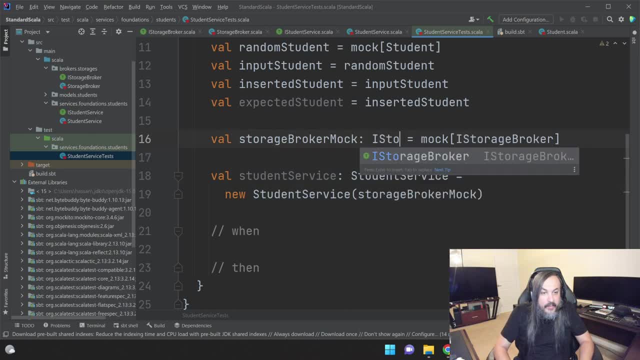 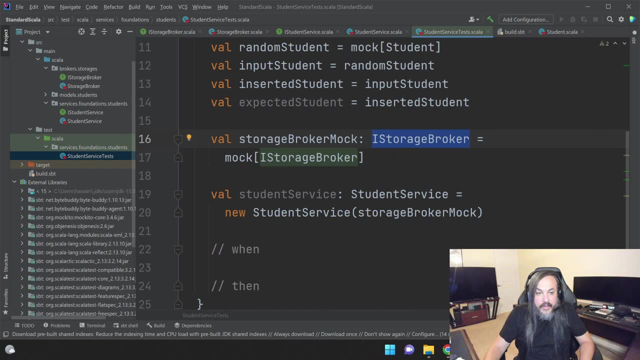 Add the type annotation, Yes, please. And also in here I want to add the type annotation. If I say I storage broker here, Yeah, see, it doesn't care if this is a mocked object, because it still honors the same, the same type. 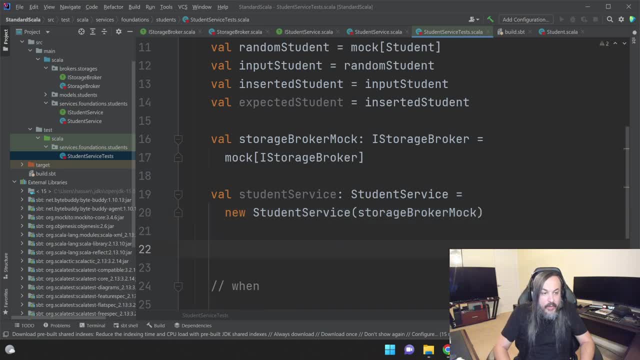 Okay, Now what? now we need to set up our thing. So our storage broker Mock. So I need to say: when storage broker mock dot, insert student with input student, then go ahead and return. We need a, we need a dependency here. What are we pulling, Makito? 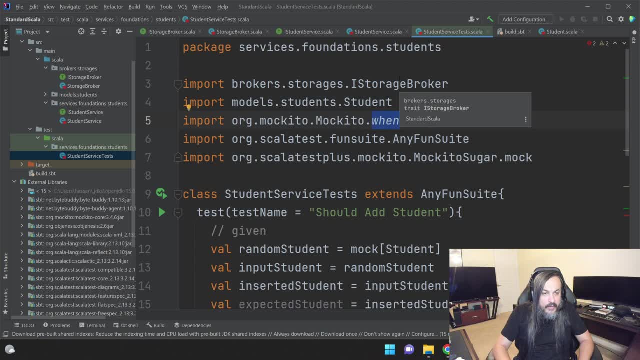 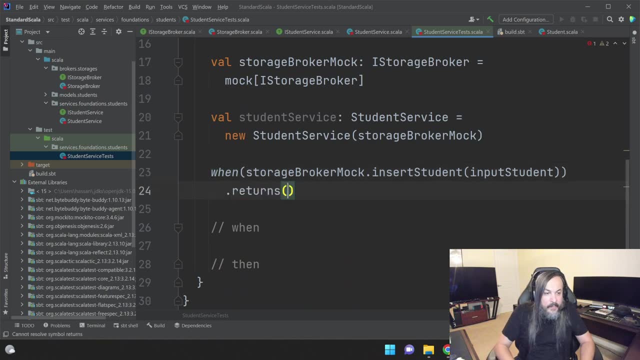 Okay, so see all of this Makito stuff. If I do this, that should just save me, but I think it's like a lot of dependencies, I guess it's. I think it's trying to be smart, so returns, and then this is inserted. 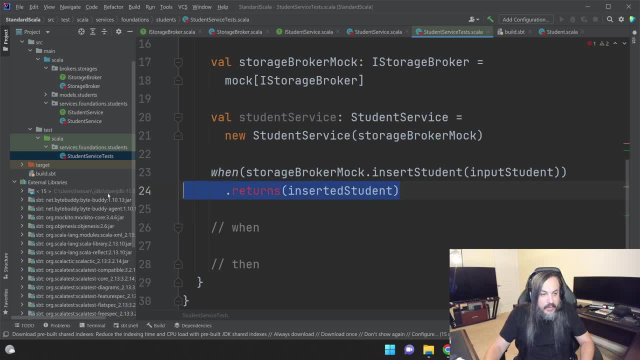 Student. I think that's how you do it. I'm not mistaken, All aware. return, Let's see, then return, then return, and then this is inserted: student. So that's your mocked area. So we just just like that, We basically mocked that. when this is passed, you have this cool. 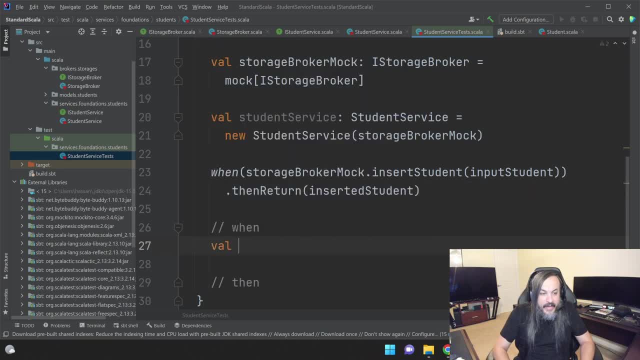 So far, so good. Now let's test this. You have Val actual student equals. And then this is your student model. And then I want to call my student service Dot add student with input student. So this is my actual student. 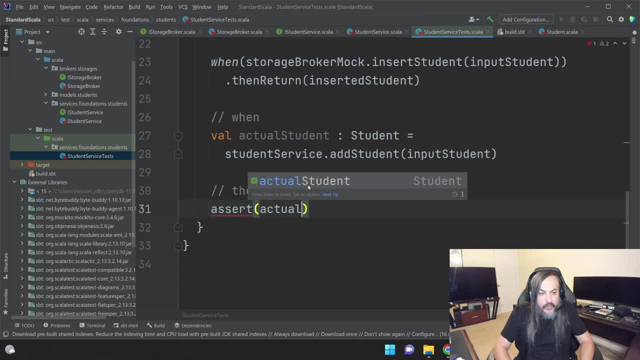 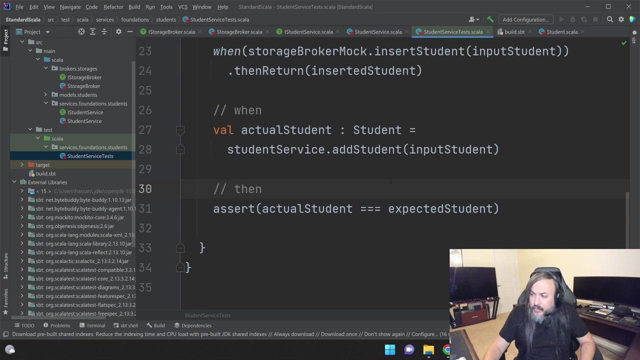 Now I can go and say: assert Actual student equal, equal Expected student. Okay, it's very straightforward, No problem there, right? Scala also has equal, equal, equal, like JavaScript, Right. And I think equal, equal, equal in Scala is the reference comparison versus the. 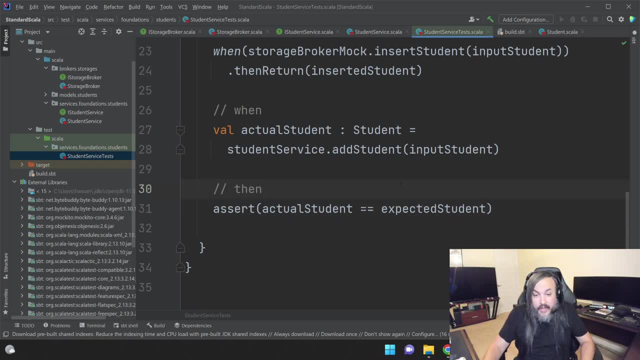 value comparison. I think that's sweet. I don't know if that's true, I don't remember, but I think that's pretty sweet because in C sharp you have to go find another library to kind of compare the value versus comparing the references, which is kind of annoying. 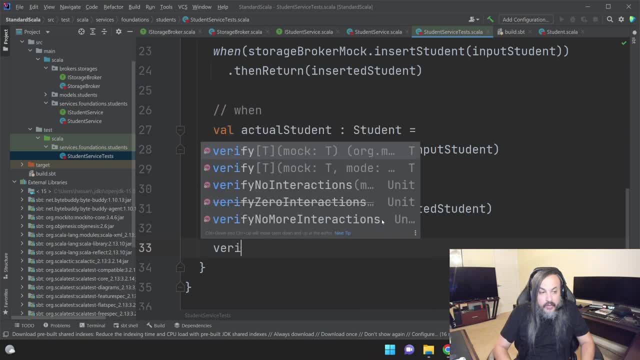 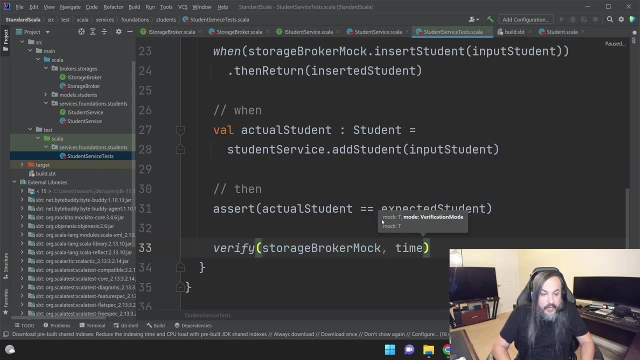 So points there for Scala also. I want to now verify. So I'm going to go here and say verify, and then here is your Storage broker- mock dot times, I think once. so that's been called once. I'll tell you what I think about this. 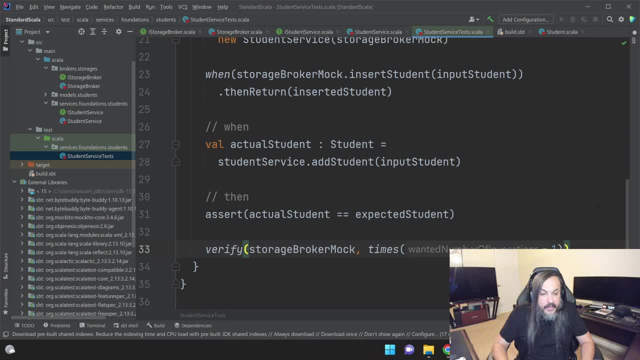 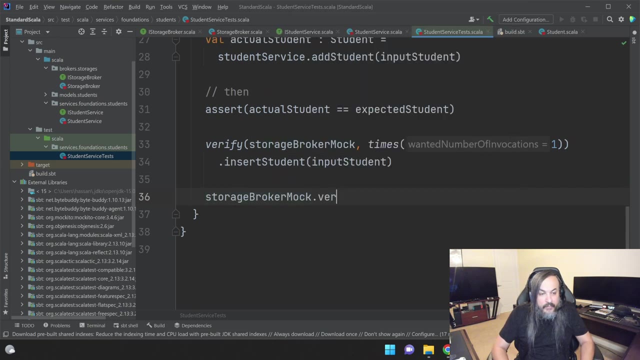 part very shortly, and then you basically go and say: dot insert student with input student. So this is my verify, So this is my way of basically in C sharp, of going and saying: storage broker, mock dot, verify Right, And here's your broker. 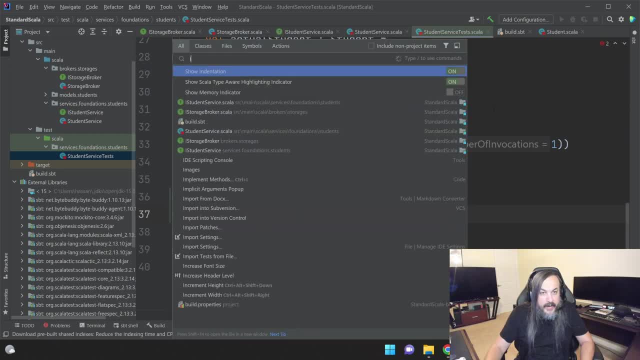 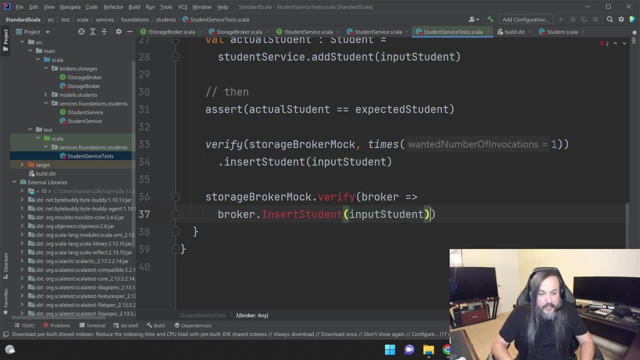 And then you go and say broker dot, what happened? broker dot, insert student input, student right times once, like this. There must be a way here in Scala where you can go and say times once as well. I'm not sure I don't remember, but this is this guy here- is basically the equivalent of this. 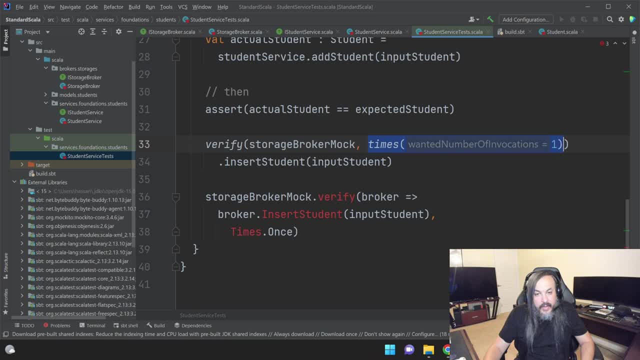 Right. I don't know if putting the times at the top here before you actually Call this. I don't like that, but that's a. I think that's a Makito thing. I think we can work around that in Scala probably. 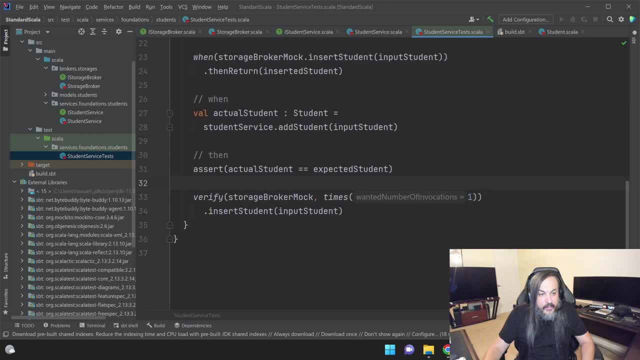 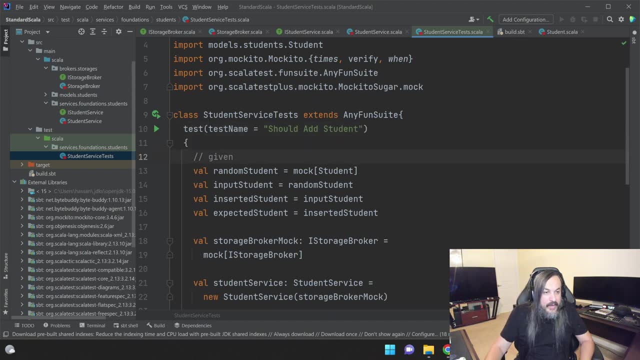 I'm not sure. Okay, so that's a failing test, my friend. So I basically going and saying This is my friends, here is all the tests that we need, And I think that should be good. Let's go run these tests and see what happens. 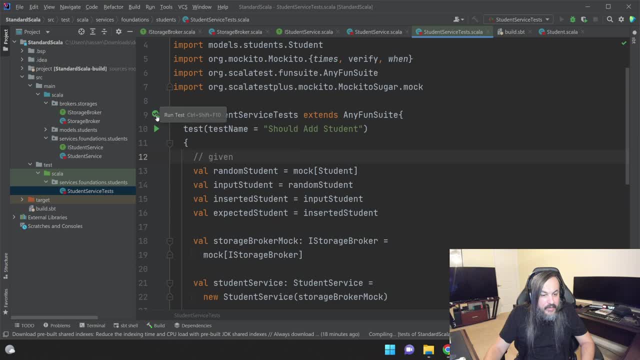 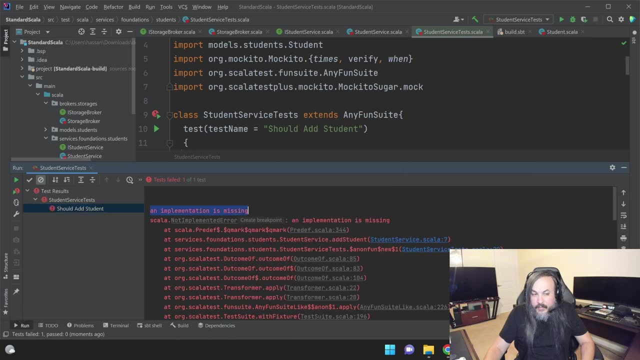 Run. I don't know why. is this saying green? Maybe it's it's a build Thing, it should fail. Yeah, there you go. The failure here is not, so it's basically saying an implementation is missing, Which is sweet, because all what we have in there is just these three question marks. 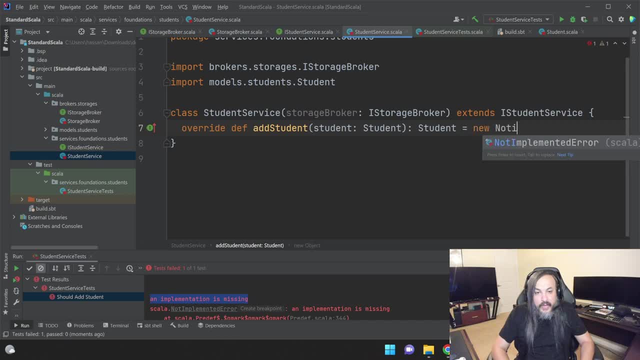 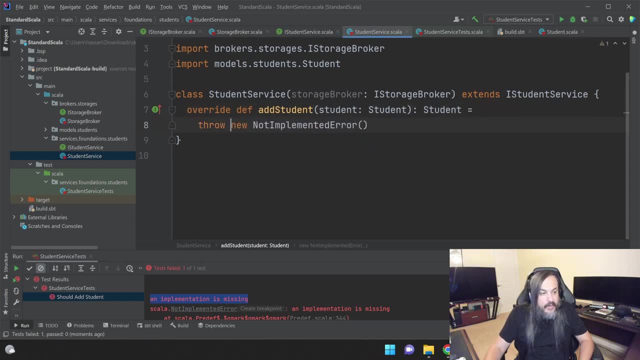 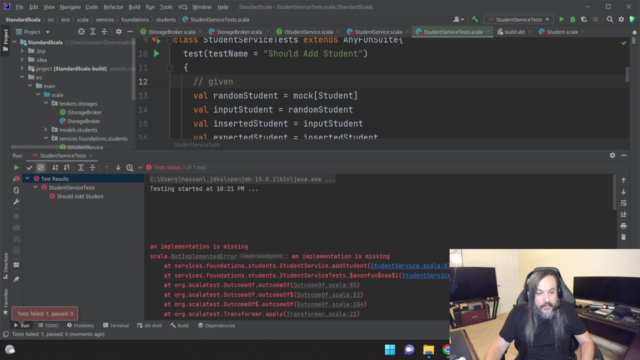 So these question marks are the equivalent of you going and saying new, not implemented error. And I think, throw new something like that, Throw new not implemented error- that you'll get the exact same problem If you run like this, There you go. So the exact same. 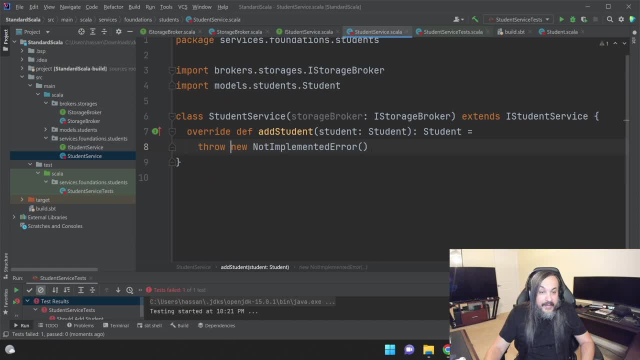 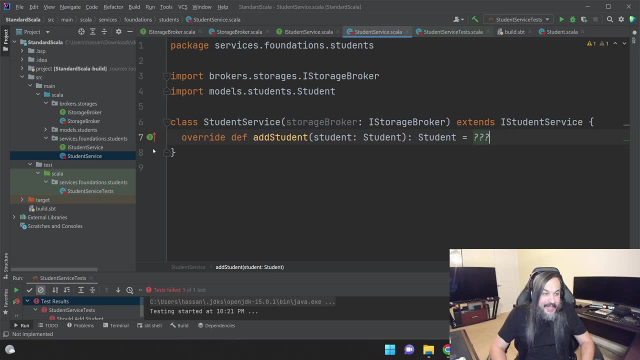 Same problem. no problem there, right? So that's again points for Scala. You know, you can just go and do this and say that's not implemented. exception: right, That's awesome, It's you, It's a. it's a really artistic way of expressing not being able to. 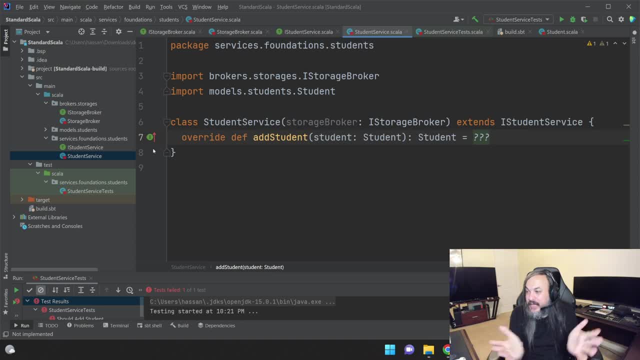 To. it's an artistic way of saying there's nothing here. yet I don't have thoughts about this yet. So, question mark, question mark, question mark. It's pretty cool, Okay. So what are we going to do here? We're going to write a function and this function will be returned. 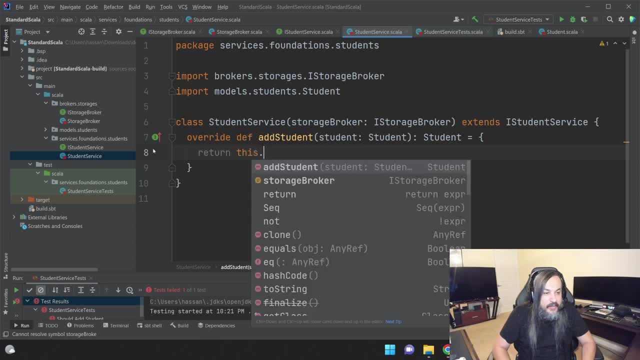 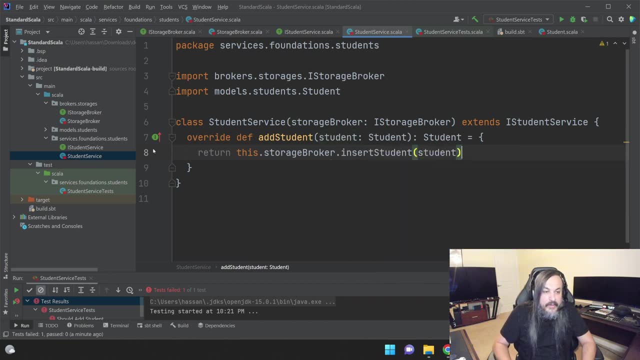 There's no. this It's storage broker. Can I actually do this? Let's see this dot who I can nice dot insert. and then this is the student Sweet. and of course the ID is telling you you don't need return. dude, It doesn't mean anything in here because it's it's trying to do as little talking as possible. 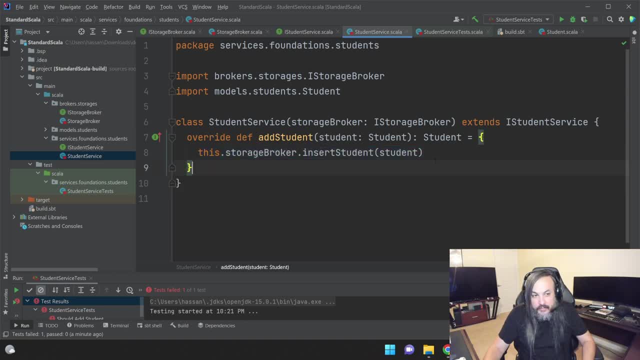 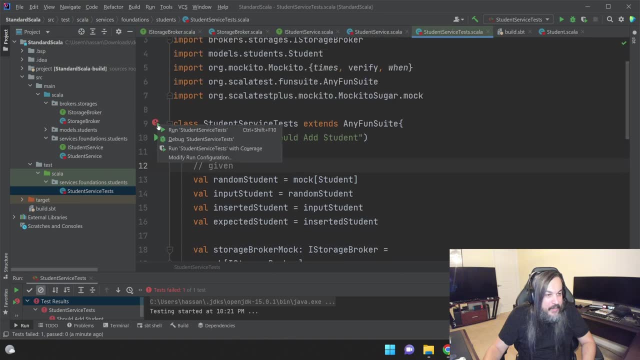 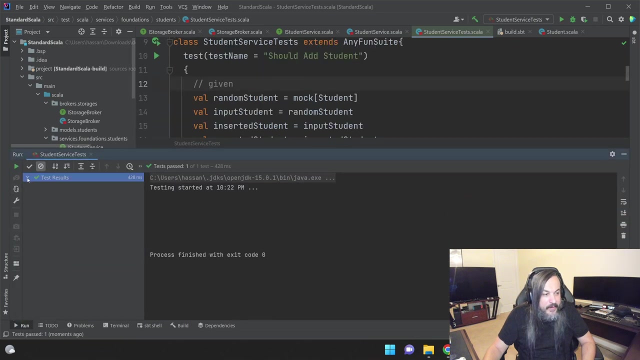 So it basically considers the last statement as vast statement, right? So let's go here and run this test again. That should pass, I think. there you go. So that's a pass, right? Here's my test. Here's my. I don't know, honestly, why it's not showing. 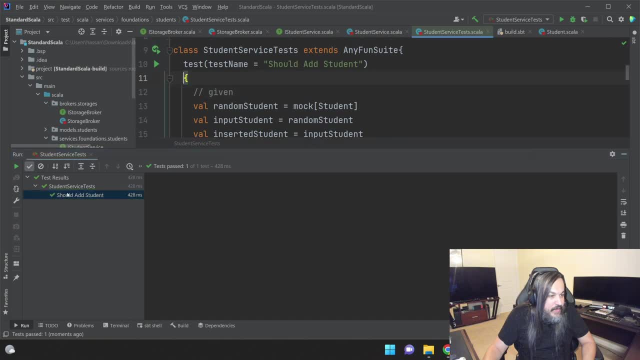 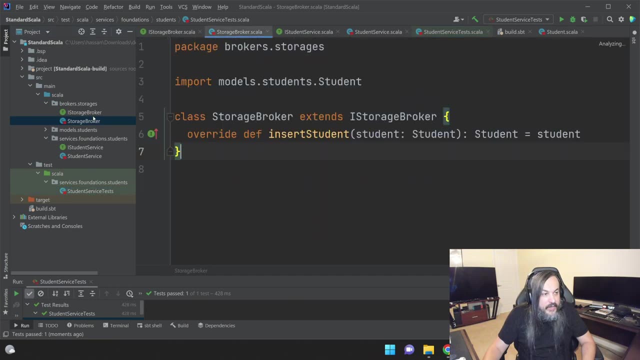 Let's see. Oh yeah, So you're basically showing failing versus passing. Yeah, I should add students. very sweet, It shows you everything you need to See. this is a very standard, friendly programming language, right? So if you're trying to implement the standard and you want to use Scala, it's definitely. 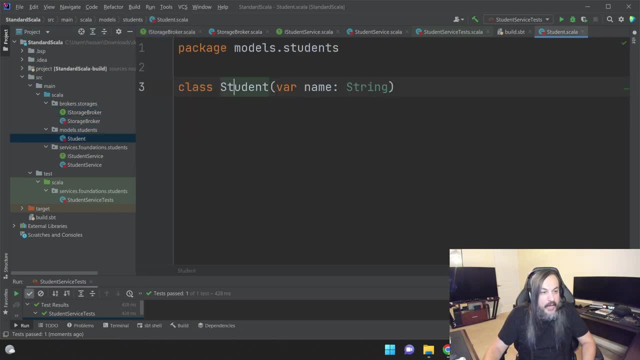 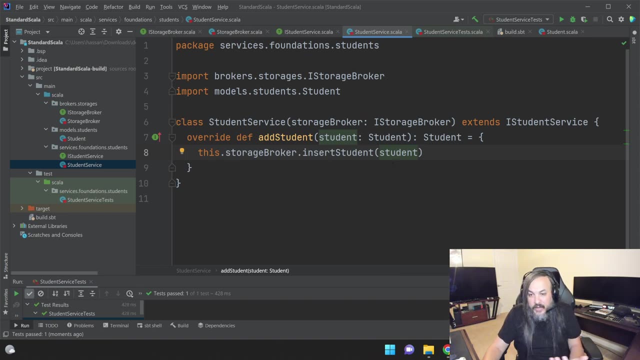 a simple again. the origins of the standard and how I started kind of building these ideas came from, you know, working a lot with functional programming languages, learning from a lot of people that you know have this kind of heart to kind of allow me to learn something. 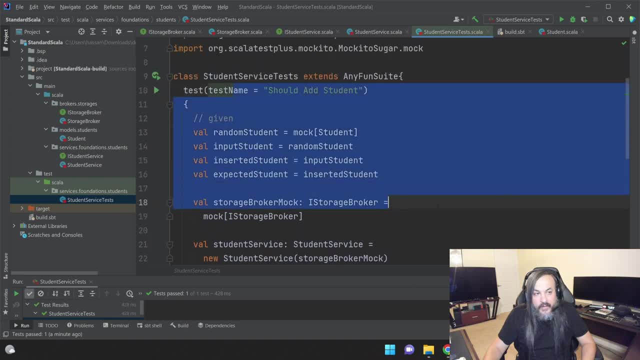 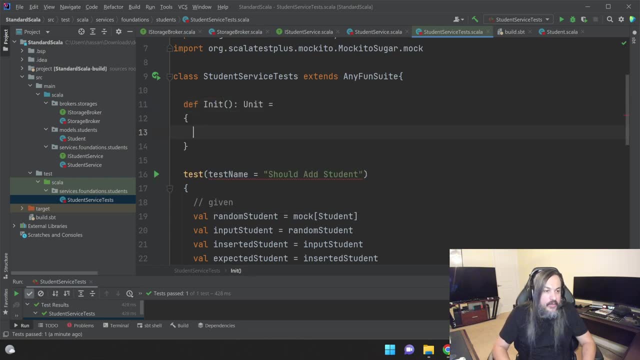 like that and, you know, build on top of it Very simple language. I think there got to be a way here where you can go and say: I don't know if is it in it or something like that, and then you basically go and say: I want to initialize the service and the broker. the same. 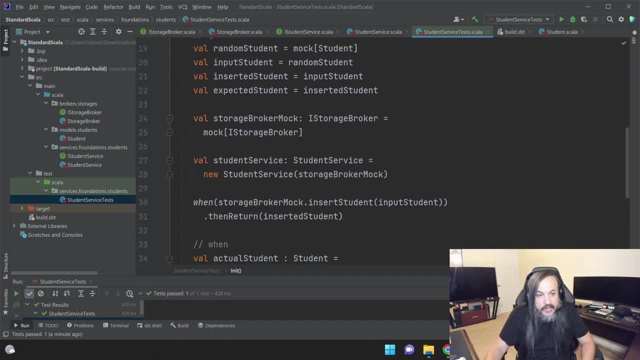 way we do it in C sharp, so you don't have to reinitialize them in here. This is this here is really dumb. We should- we should- initialize these every run with the test. There is probably a way to do it. That's not. that's not the point of this. 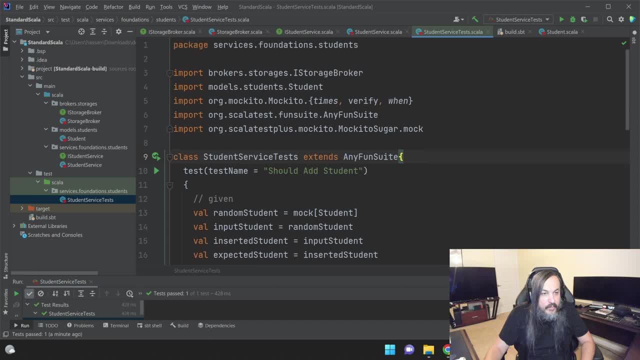 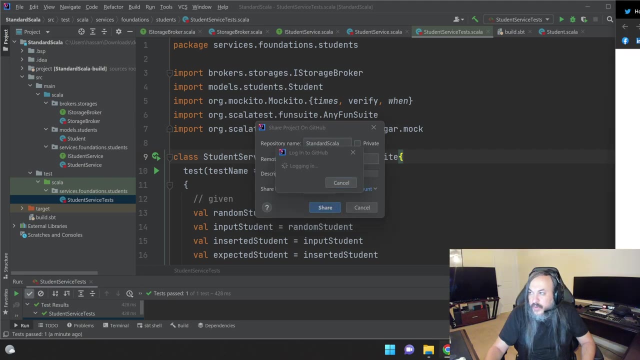 Anyway, I'm going to give you this code, kind of if you. if you never played With Scala before, this is definitely a great place to start. here is VCS share project on GitHub standard Scala origin as shared by add account login via GitHub Sure. 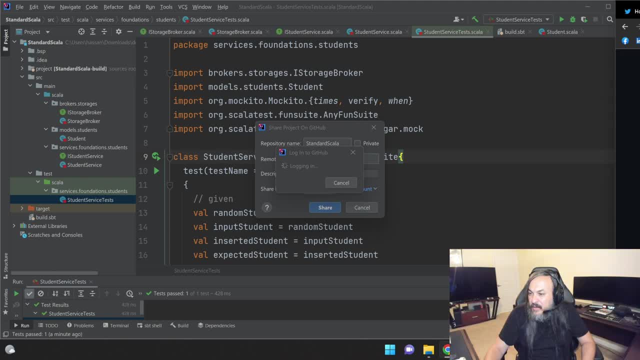 Why not? This thing is going to make me continue. See here, Yep, You have been successfully authorized, because I'm literally living on GitHub. So this is origin. This is not Private description. example demo project in Scala to implement the standard. 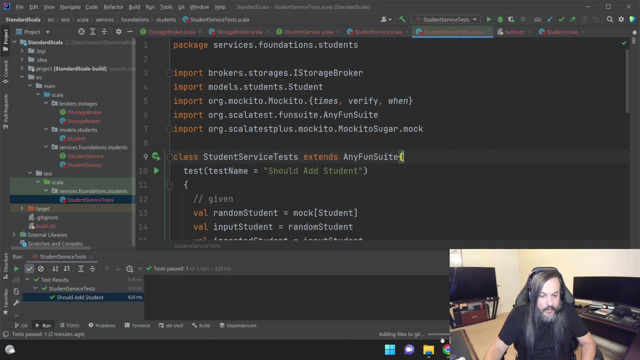 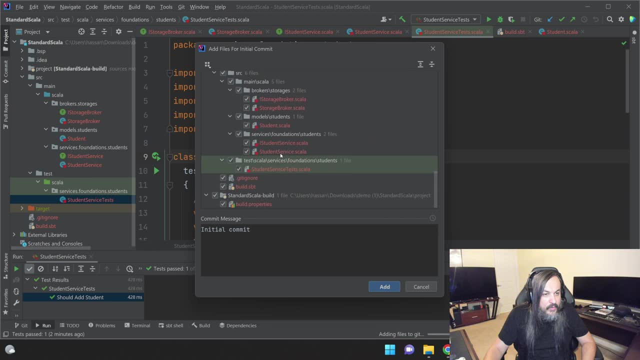 Okay, so I'm sharing this project out here. You should be able. Let's see here. Wow, I'll call these things. I don't think we need idea stuff in here or the libraries, You just need the source code. Yeah, it should be smart enough to do this. 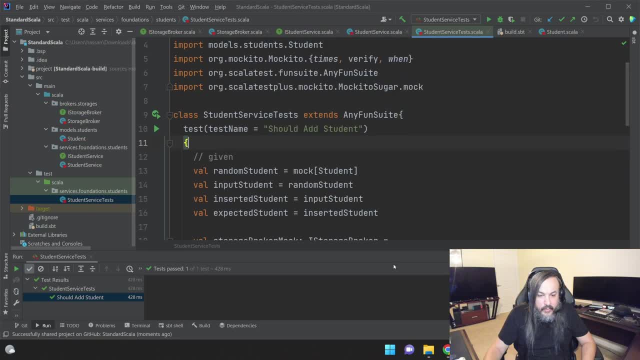 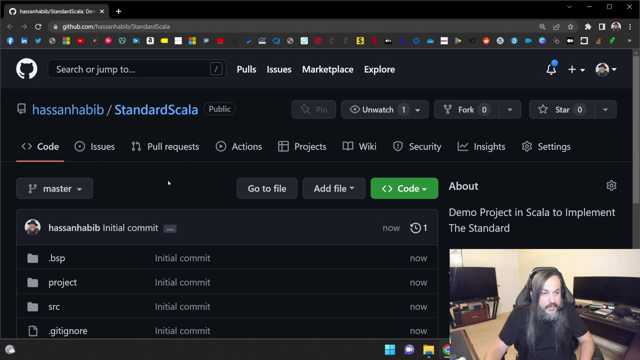 Here you go: Add: Here's your Scala program, right there. So now, if I click on this, it should open up a new page for you. It should basically tell you: here is your Scala app Right. So I'm going to add the. read me here. 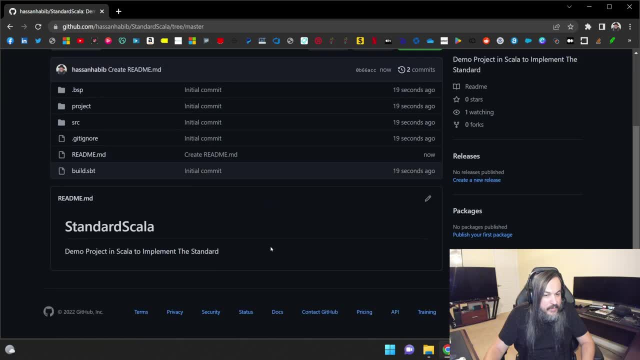 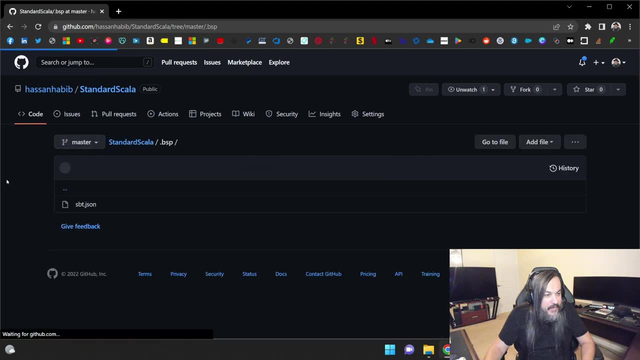 I'm going to say: this is a demo for Scala. There you go, Beautiful, right, You have everything, and I don't think I should have added this BS, BSP as well. Whatever that is. Oh, that's know that I would probably need that. 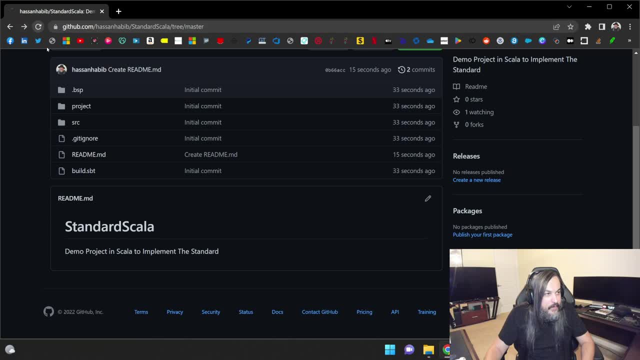 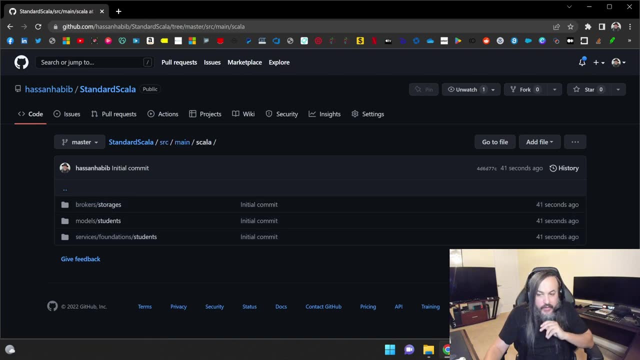 I don't know. I think it's a jet brains thing. Okay, so this is that beautiful language you know. take a look, See. you know how the language works. It's very, very, very easy to implement certain ideas in this language. 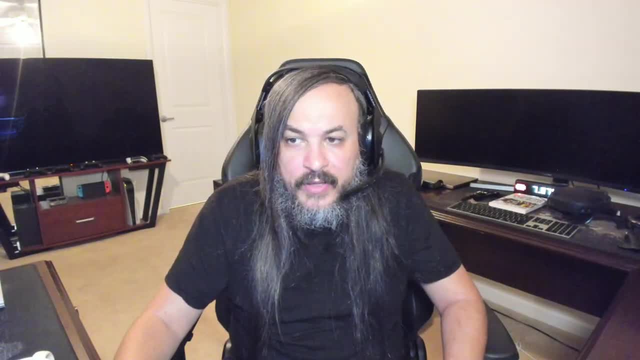 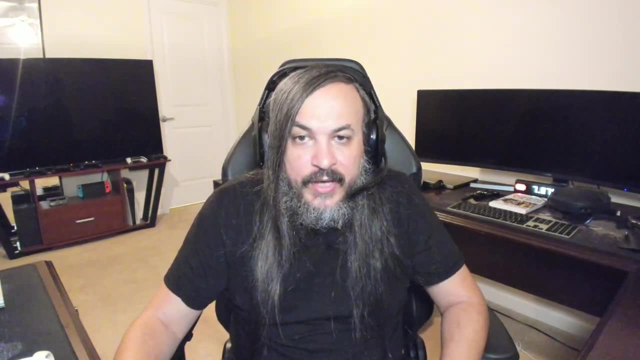 Very easy to kind of bring you know your thoughts. It'll teach you a lot of things. It has some superiority in terms of certain implementations. It has some superiority when it comes to It makes you think like a functional as programming language of you know. 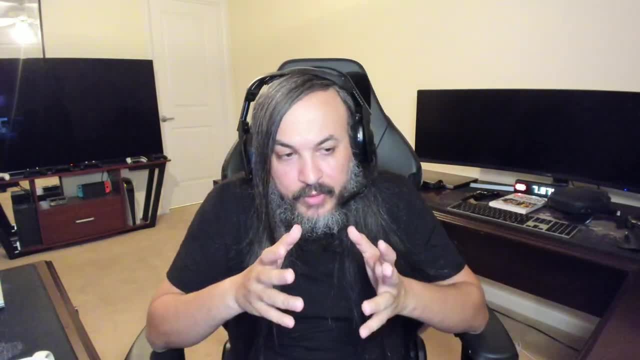 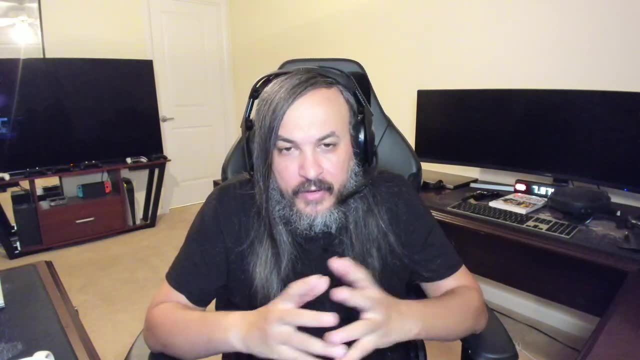 it's a software scientist, but it also, more importantly, it has a lot of nice tricks. You know there's for comprehension, There's pattern matching, a lot of crazy stuff. You know you can do a synchronous thing. I think use future. you know so many different things. 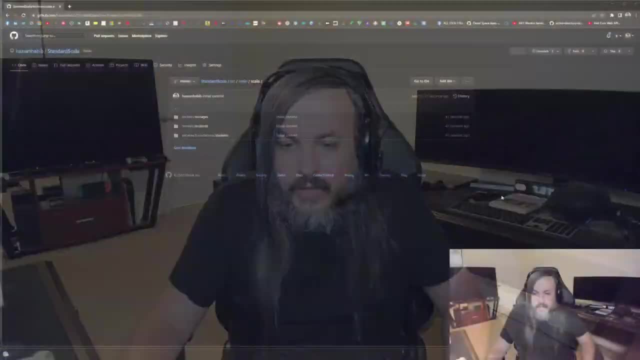 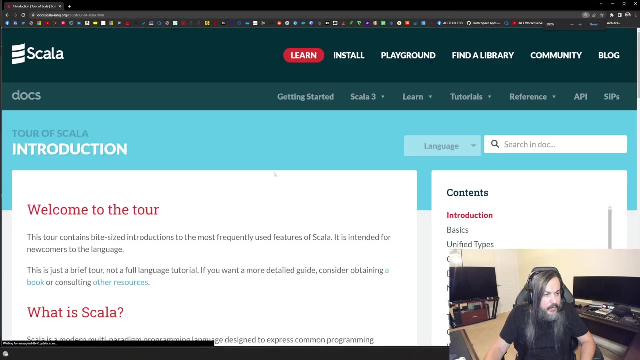 Where do you, where do you find all these things about Scala? If you look at, if you just say tour and Scala, which is basically where I was kind of refreshing My memory on it, you'll find all kinds of nice stuff in here. 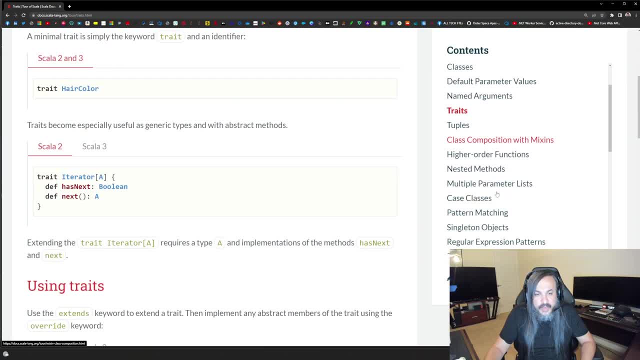 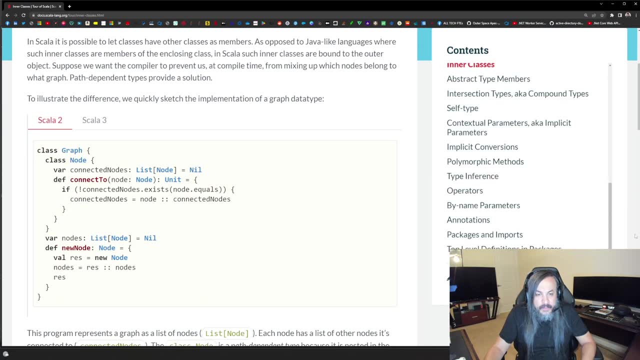 It has traits. Traits are basically interfaces. I'll drop that. I'll drop that link over in the description as well. So you can see. you can see inner grasses, classes, But then again you know, such as the case with every programming language or technology, about the community, right. 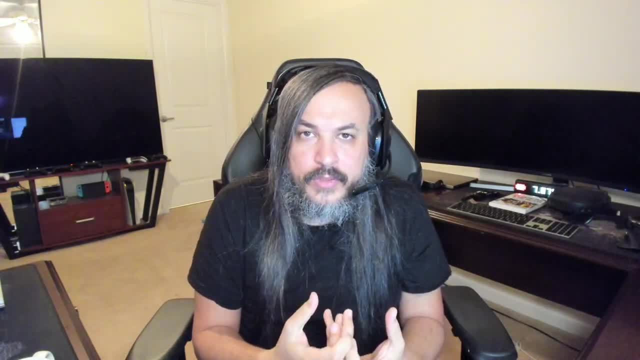 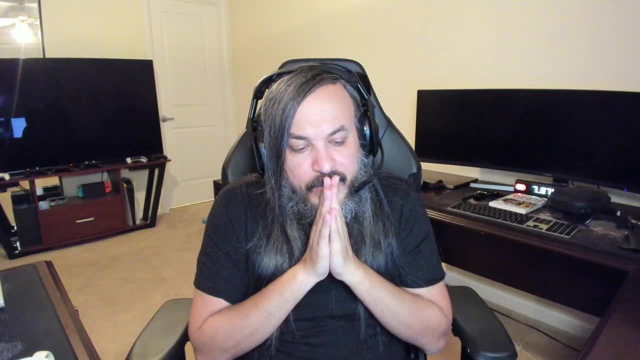 You know how much people are building. you know libraries that can support. you know what, if you want to add security, How hard is it to add security? You know they have a thing I think called Was it sprites or something like that. 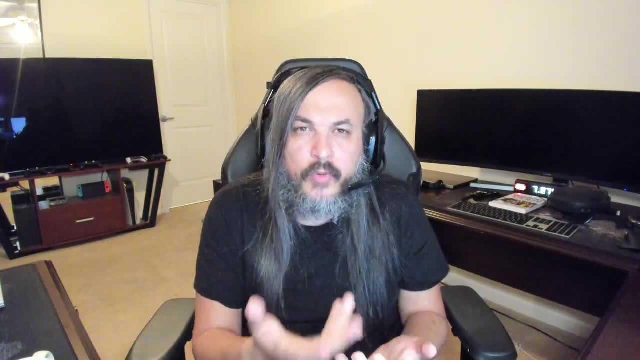 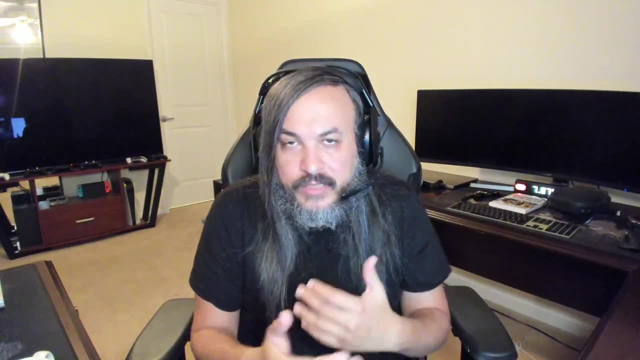 It's the equivalent of the entity framework, right? You basically go and say, or spark or something like that: for the most part, Scala is being used for big data stuff. right, You're doing data processing and stuff like that. Go to Scala. 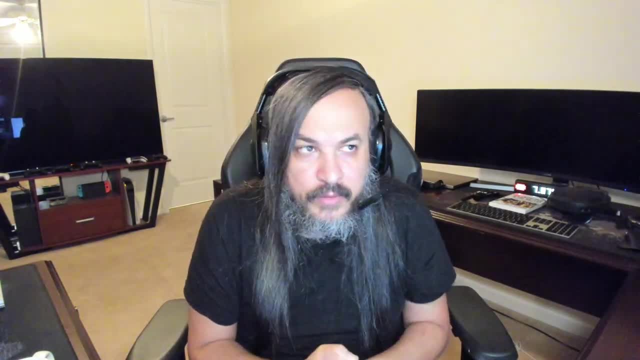 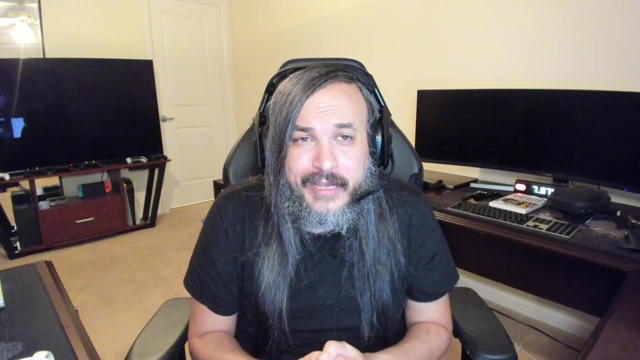 It's great, but you can use it as a general programming language. You can build, you know, api's and stuff like that. I hope you find this useful. I hope you find this kind of a little bit eye-opening in terms of how to build systems. 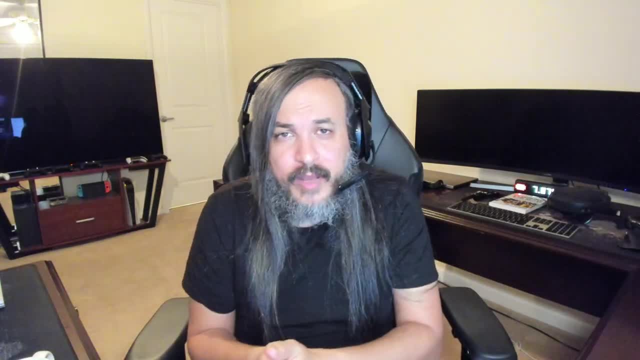 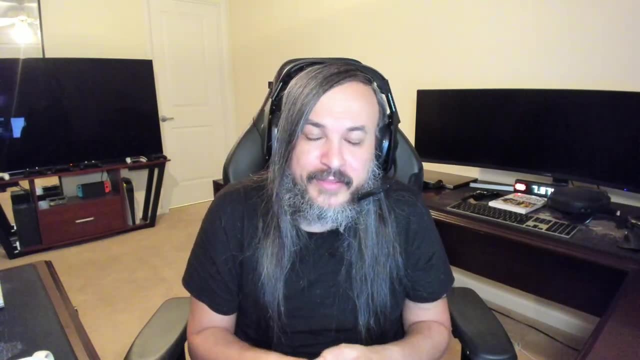 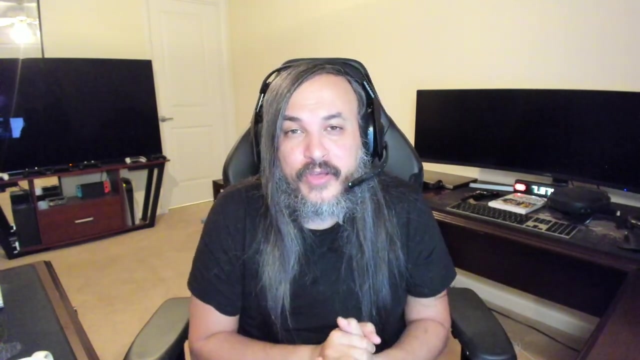 You know a standard compliance systems in different programming languages. I'll continue to kind of explore different languages. I'm still fighting with rust a little bit. Maybe we can do it in C++, Maybe we can do it in Java. It's going to be the easiest and jobs a little chatty, but it's going to be a lot similar to Scala when it comes to Java. 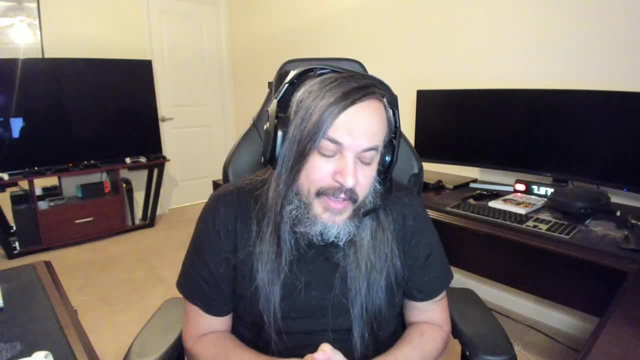 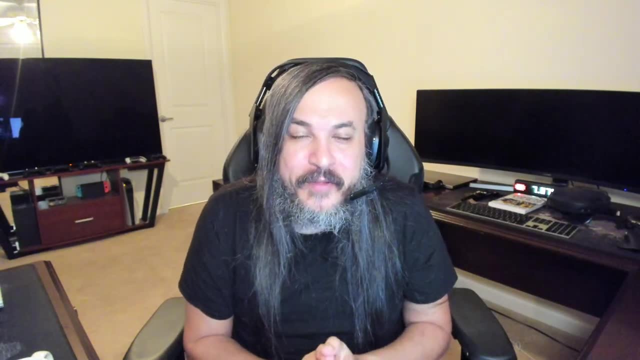 Maybe Kotlin, maybe some of these programming languages. We'll see how things go, I hope. I hope that this is a useful content for you And if you have any questions, comments concerns, please feel free, Drop comments in the comment section and don't forget to like and subscribe.